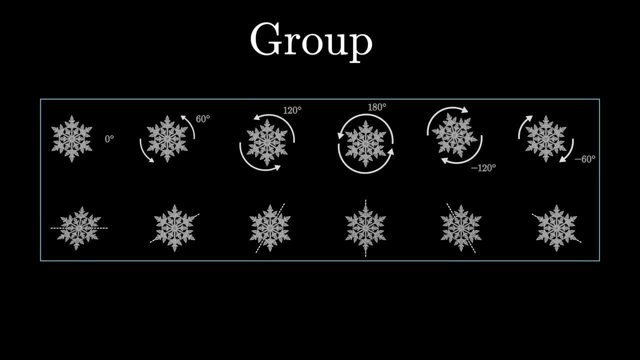 Take note, the fact that mathematicians have co-opted such an otherwise generic word for this seemingly-specific kind of collection should give you some sense of how fundamental they find it. 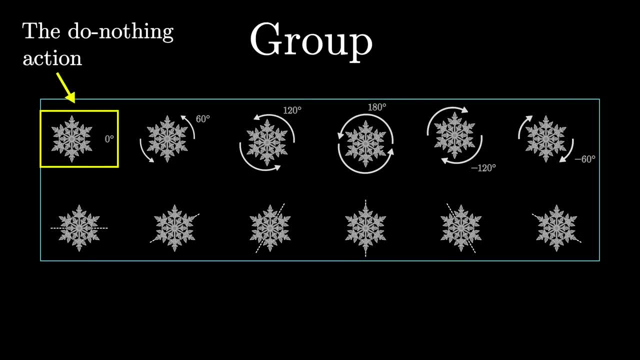 Also, take note, we always consider the action of doing nothing to be part of the group. So if we include that do-nothing action, the group of symmetries of a snowflake includes 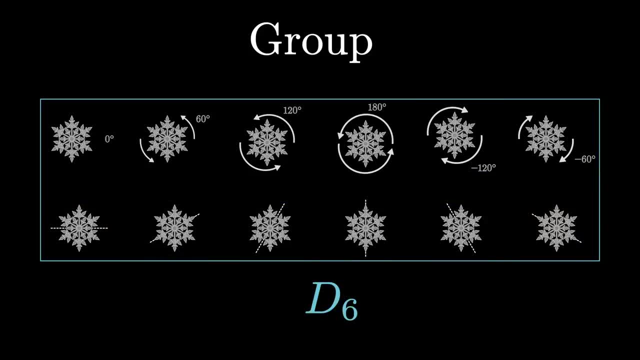 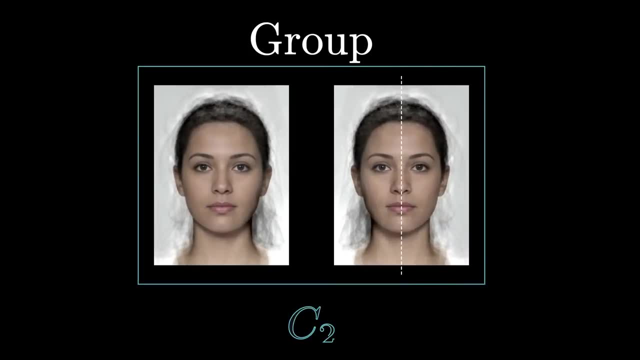 12 distinct actions. It even has a fancy name, D6. The simple group of symmetries that only has two elements acting on a single action. on a face also has a fancy name, C2. In general, there is a whole zoo of groups with no shortage 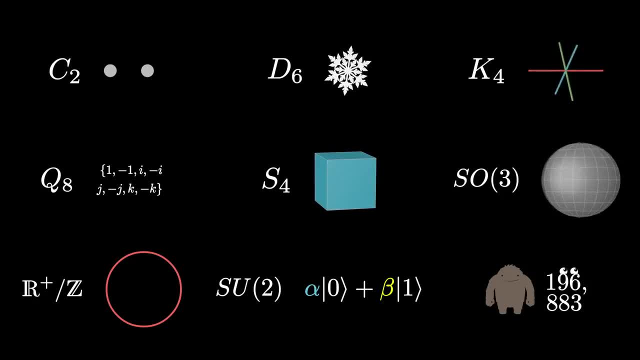 of jargon to their names categorizing the many different ways that something can be symmetric. 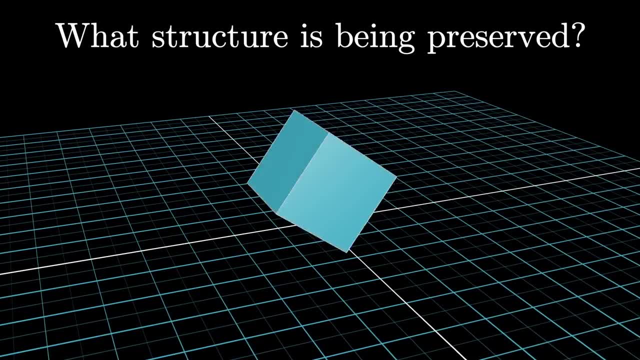 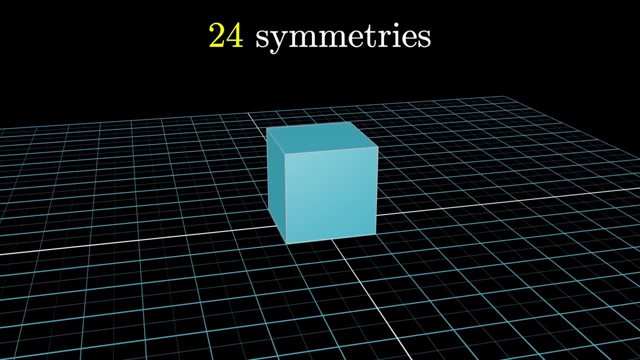 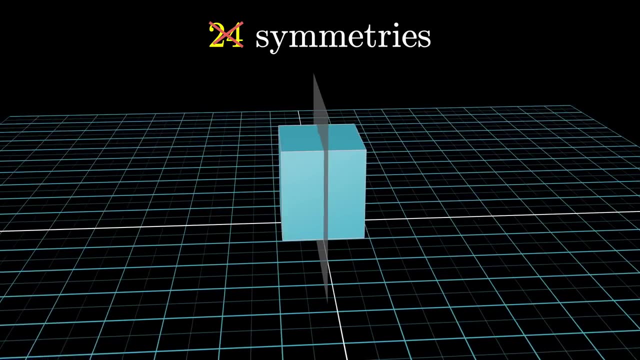 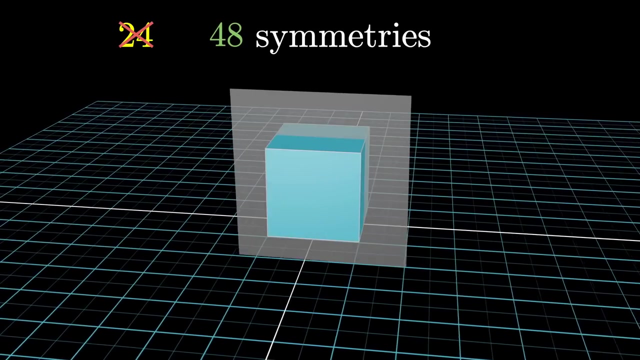 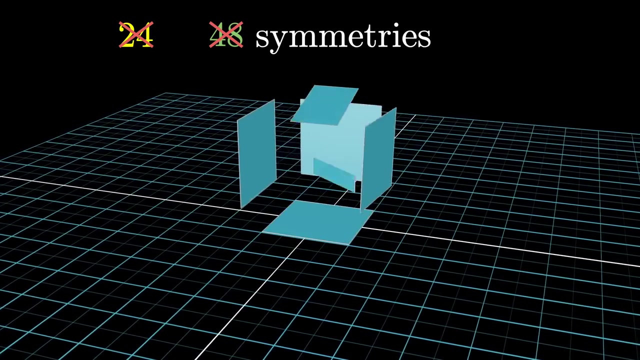 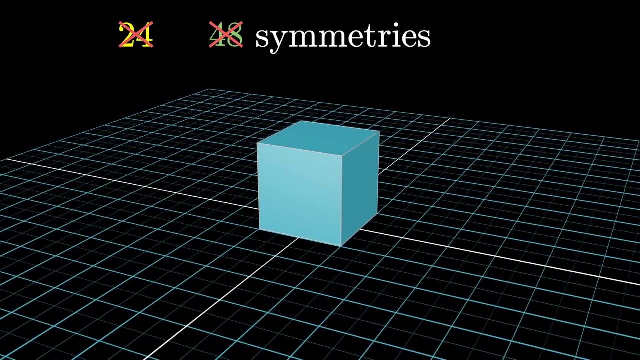 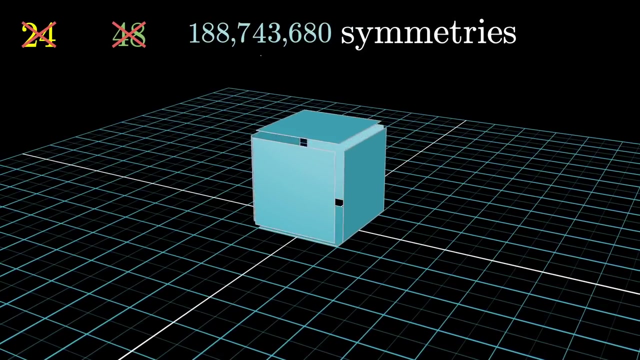 When we describe these sorts of actions, there's always an implicit structure being preserved. For example, there are 24 rotations that I can apply to a cube that leave it looking the same, and those 24 actions taken together do indeed constitute a group. But if we allow for reflections, which is a kind of way of saying that the orientation of the cube is not part of the structure we intend to preserve, you get a bigger group with 48 actions in total. If you loosen things further and consider the faces to be a little less rigidly attached, maybe free to rotate and get shuffled around, you would get a much larger set of actions. And yes, you could consider these symmetries in the sense that they leave it looking the same, and all of these shuffling, rotating actions do constitute a group, but it's a much bigger and more complicated group. 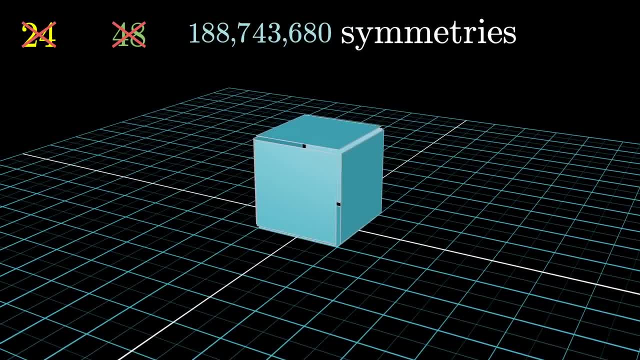 The large size in this group reflects the much looser sense of structure which each action preserves. 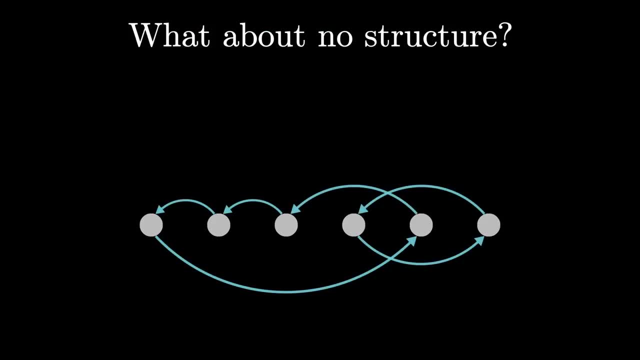 The loosest sense of structure is if we have a collection of points and we consider any way you could shuffle them, any permutation, to be a symmetry of those points. Unconstrained by any underlying property that needs to be preserved, these permutation groups can get 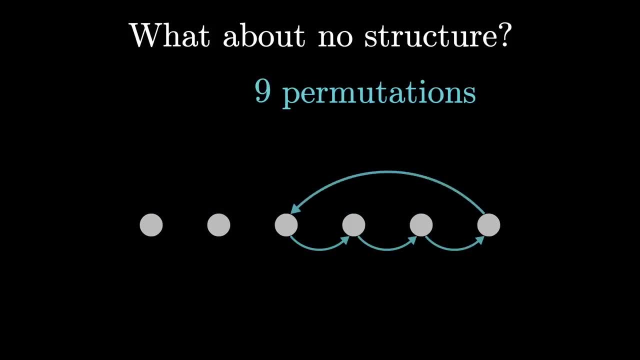 quite large. Here, it's kind of fun to flash through every possible permutation of six objects, and see how many there are. 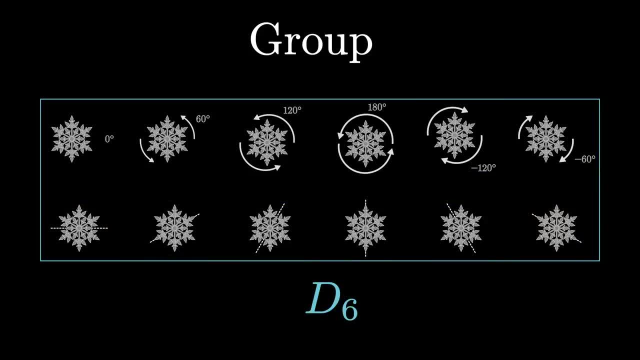 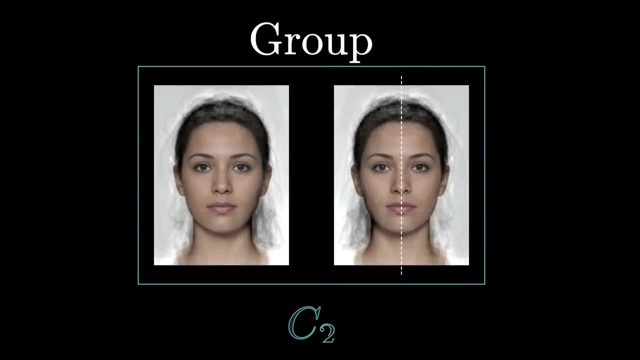 12 distinct actions. It even has a fancy name: d6.. The simple group of symmetries that only has two elements acting on a single group is called d6.. The group of the two elements acting on a face also has a fancy name: c2.. 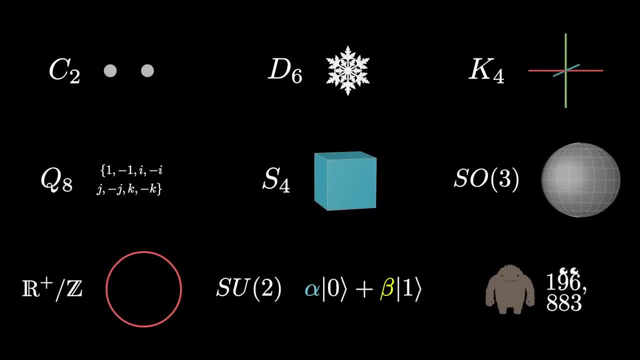 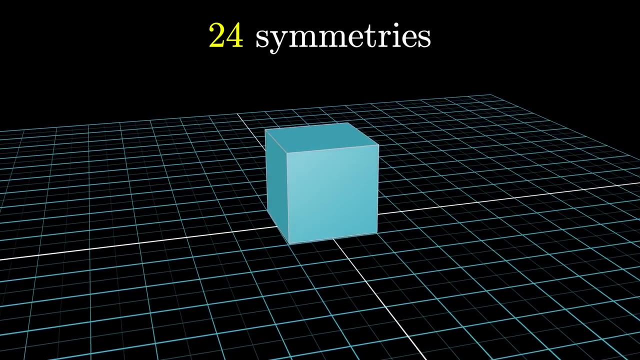 In general, there is a whole zoo of groups with no shortage of jargon to their names, categorizing the many different ways that something can be symmetric. When we describe these sorts of actions, there is always an implicit structure being preserved. For example, there are 24 rotations that I can apply to a cube. that leave it looking. 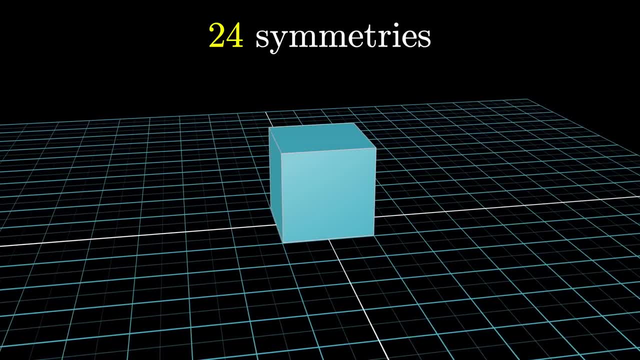 the same, And those 24 actions taken together do indeed constitute a group. But if we allow for reflections, we can also use the same term to describe a group, For example, if we consider the orientation of the cube, which is a kind of way of saying that the 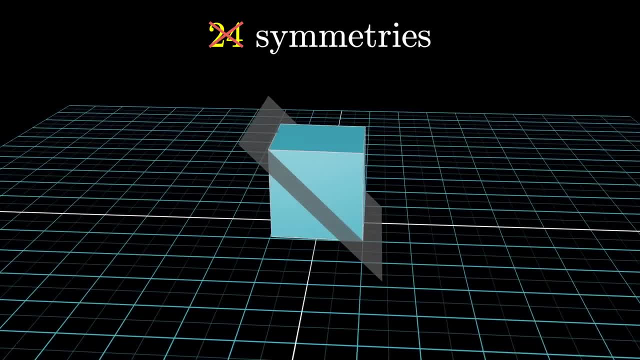 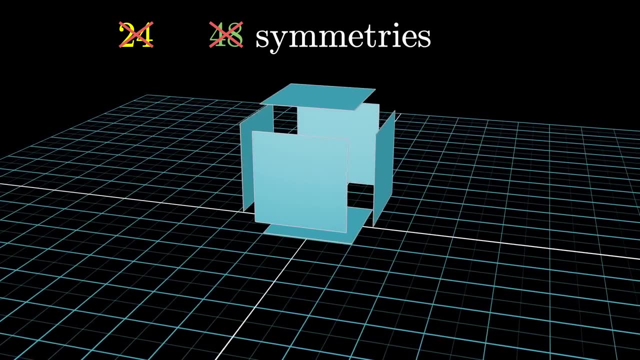 orientation of the cube is not part of the structure we intend to preserve. you get a bigger group with 48 actions in total. If you loosen things further and consider the faces to be a little less rigidly attached, maybe free to rotate and get shuffled around. 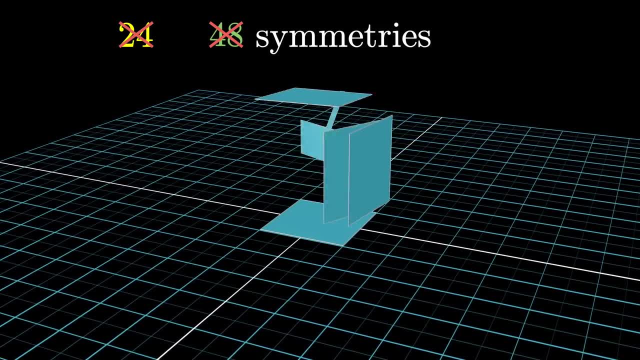 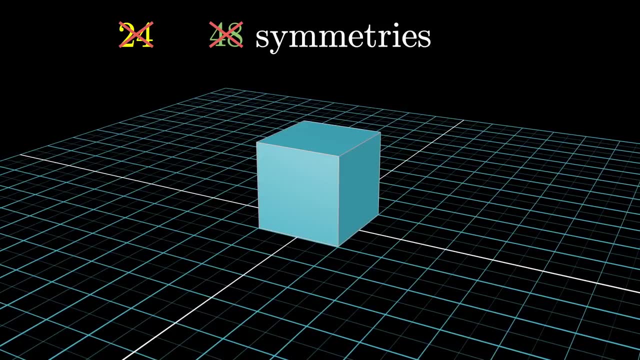 you would get a much larger set of actions. And, yes, you could consider these symmetries in the sense that they leave it looking the same and all of these shuffling, rotating actions do constitute a group, but it's a much bigger and more complicated group. 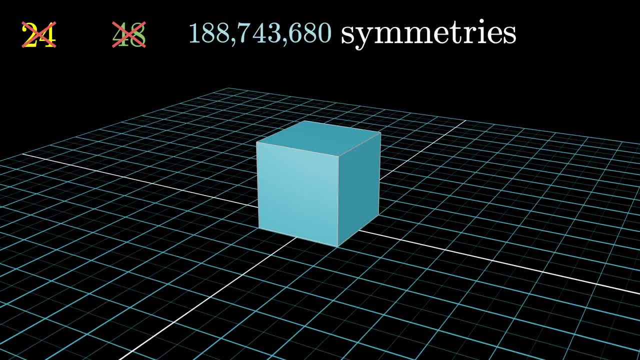 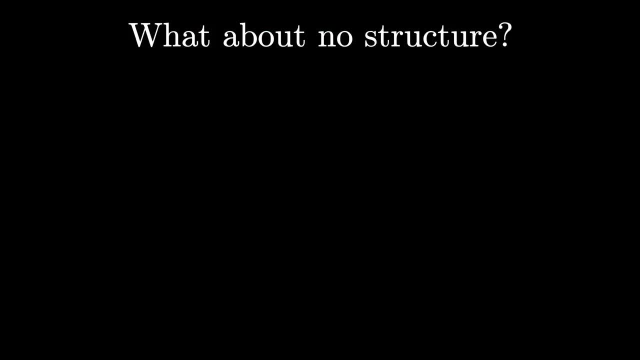 The large size in this group reflects the much looser sense of structure which each action preserves. The loosest sense of structure is if we have a collection of points and we consider, any way you could shuffle them, any permutation, to be a symmetry of those points, Unconstrained. 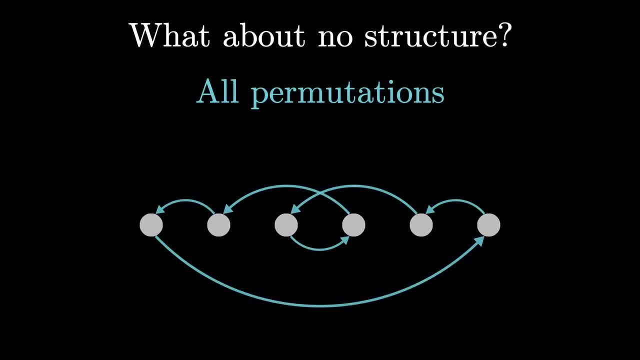 by any underlying property that needs to be preserved. these permutation groups can get quite large. Here it's kind of fun to flash through every possible permutation of 6 objects and see how many there are. In total it amounts to 6 factorial or 720.. By contrast, if we gave these points some, 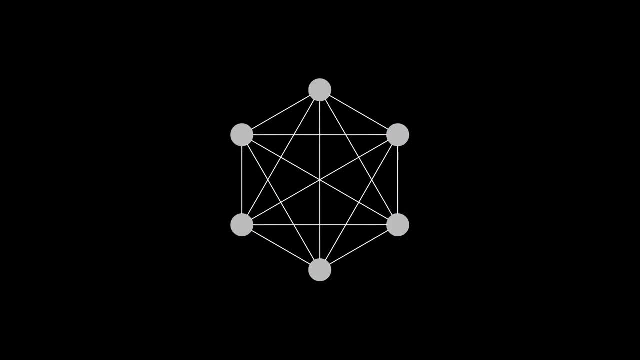 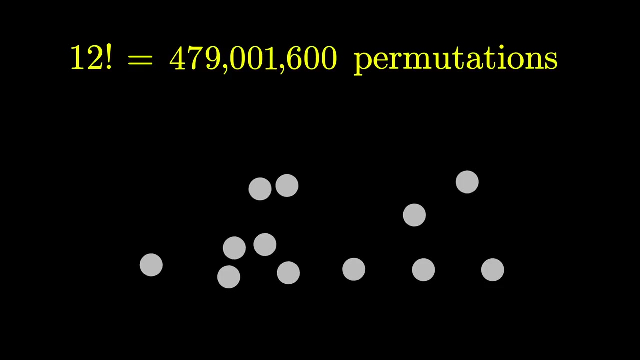 structure, maybe making them the corners of a hexagon and only considering the permutations that preserve how far apart each one is from the other. well then, we only get the 12 snowflake symmetries we saw earlier Bump the number of points up to 12, and the number of permutations grows to about 479. 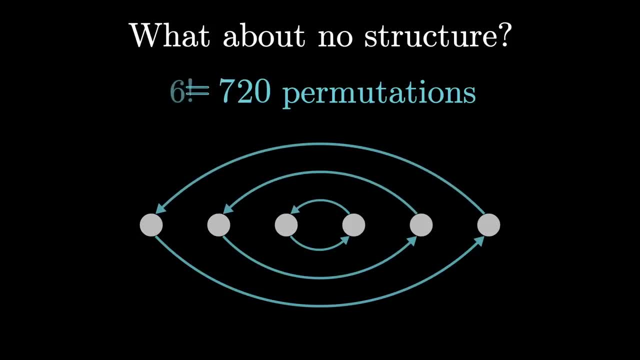 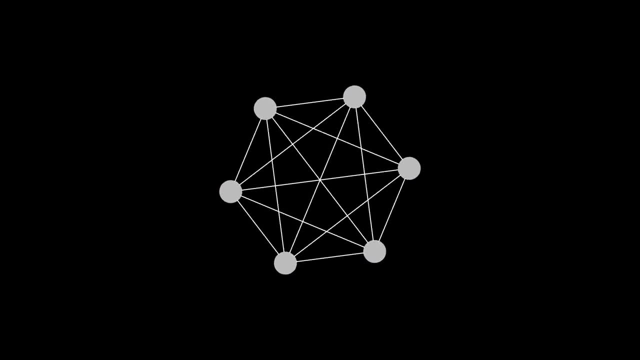 In total, it amounts to 6 factorial, or 720. By contrast, if we gave these points some structure, maybe making them the corners of a hexagon and only considering the permutations that preserve how far apart each one is from the other, well then we only get the 12 snowflake symmetries we saw. 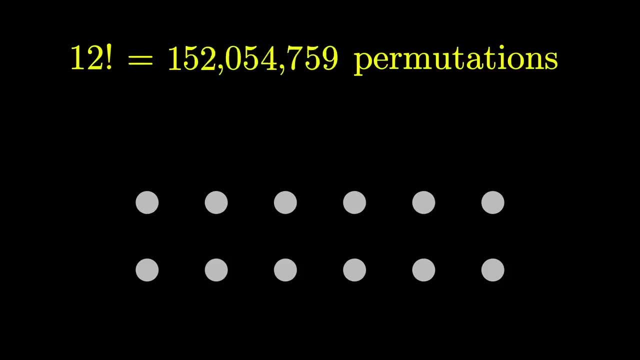 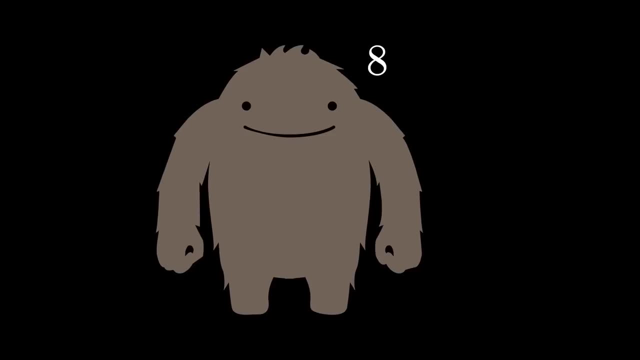 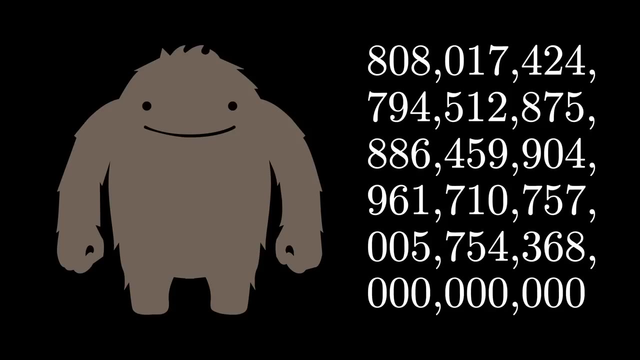 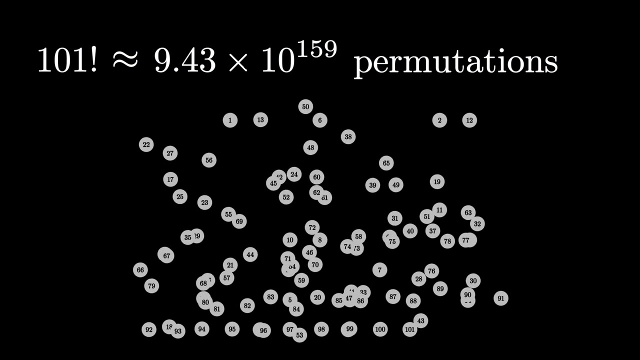 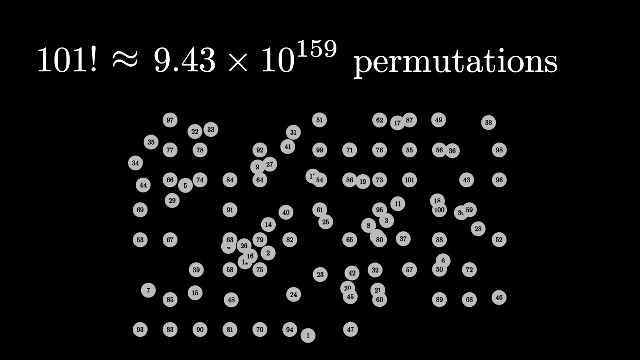 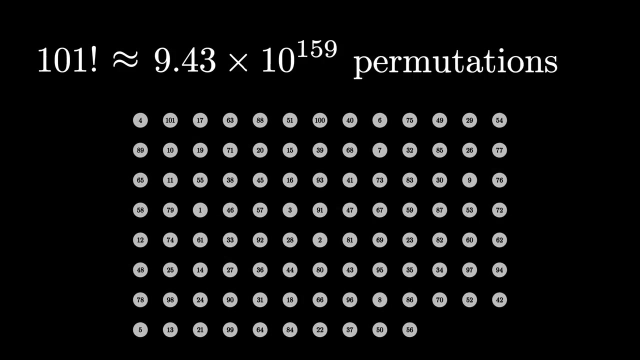 Bump the number of points up to 12, and the number of permutations grows to about 479 million. The monster that we'll get to is rather large, but it's important to understand that largeness in and of itself is not that interesting when it comes to groups. The permutation groups already make that easy to see. If we were shuffling 101 objects, for example, with the 101 factorial different actions that can do this, we have a group with a size of 9x10 to 159. If every atom in the observable universe had a copy of that universe inside itself, this is roughly how many subatoms there would be. These permutation groups go by the name S sub n, and they play a very important role in group theory. In a certain sense, they encompass all other groups. 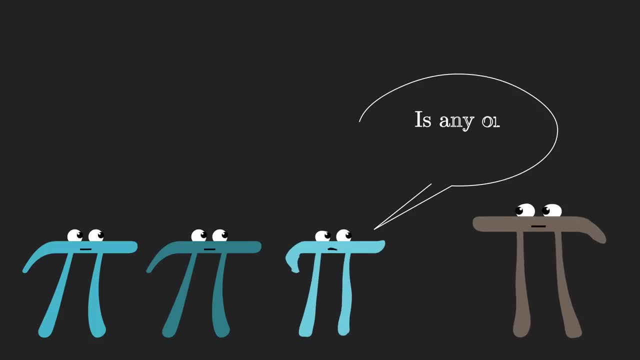 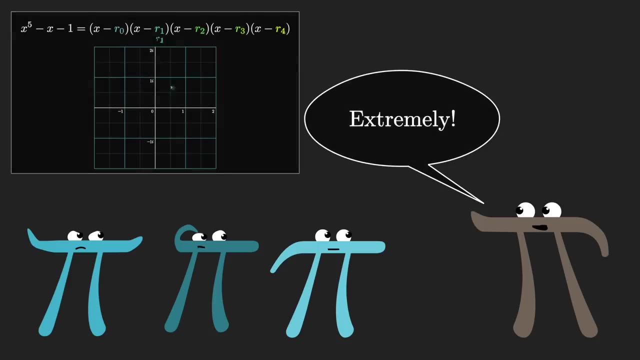 And so far, you might be thinking, okay, this is intellectually playful enough, but is any of this actually useful? One of the earliest applications of group theory came when mathematicians realized that the structure of these permutation groups tells us something about solutions to polynomial equations. 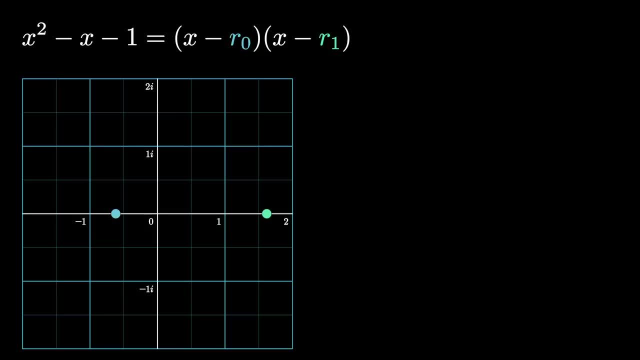 You know how in order to find the two roots of a quadratic equation, everyone learns a certain formula in school? Slightly lesser known is the fact that there's also a cubic formula, one that involves nesting cube roots with square roots in a larger expression. There's even a quartic formula for a degree four polynomial, which is an absolute mess. It's almost impossible to write without factoring things out. And for the longest time, mathematicians struggled to find a formula to solve degree five polynomials. I mean, maybe there's one, but it's just super complicated. 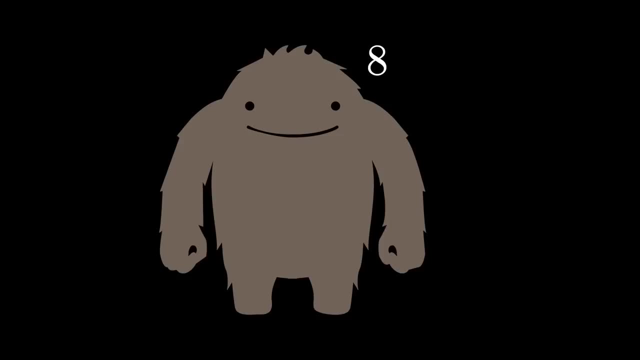 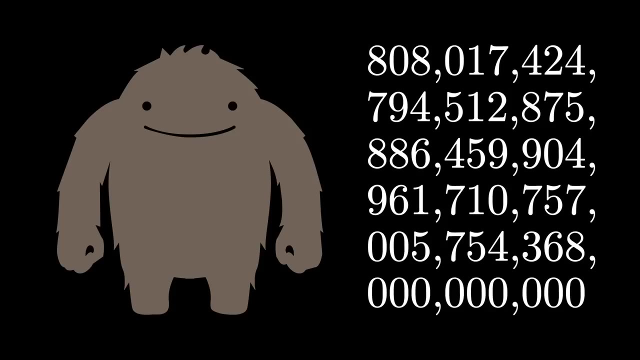 million. The monster that we'll get to is rather large, but it's important to understand that largeness in and of itself is not that interesting when it comes to groups. The permutation groups already make that easy to see. If we were shuffling 101 objects, for example, with the. 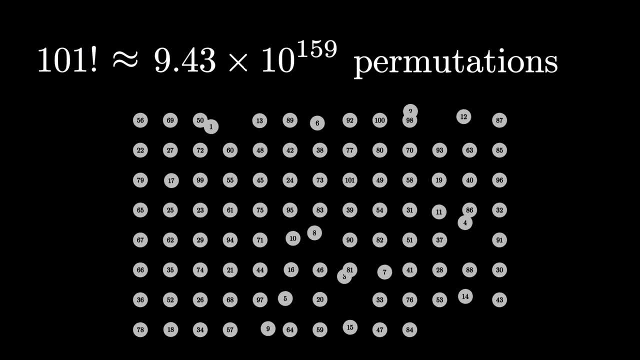 101 factorial different actions that can do this, we have a group with a size of around 9 times 10 to the 159.. If we were shuffling 101 objects, for example, with the 101 factorial different actions that can do this, we have a group with a size of around 9 times 10 to the 159.. If every atom 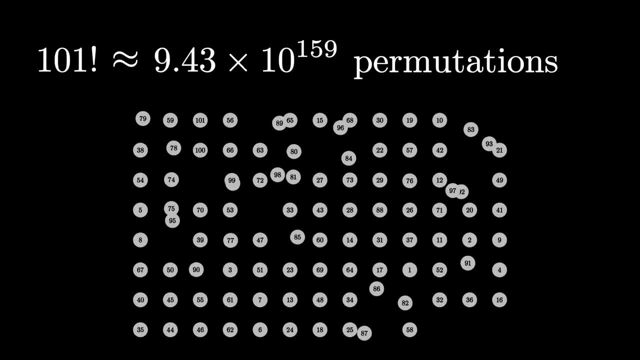 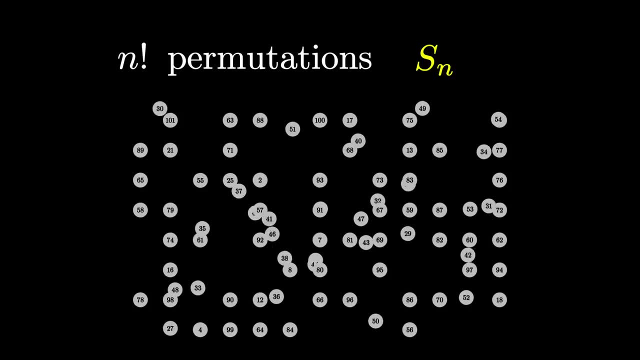 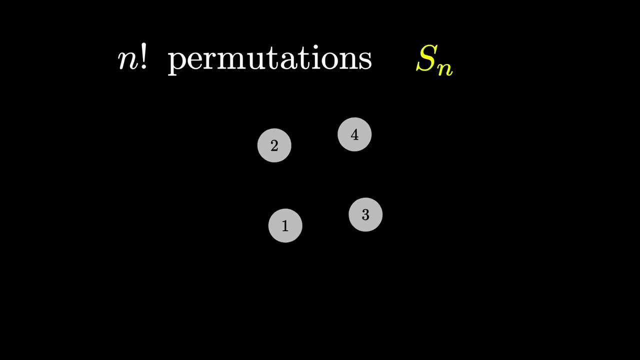 in the observable universe had a copy of that universe inside itself. this is roughly how many subatoms there would be. These permutation groups go by the name S, sub n, and they play a very important role in group theory. In a certain sense they encompass all other groups. 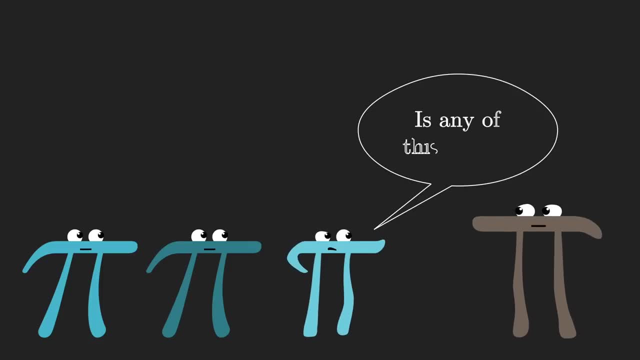 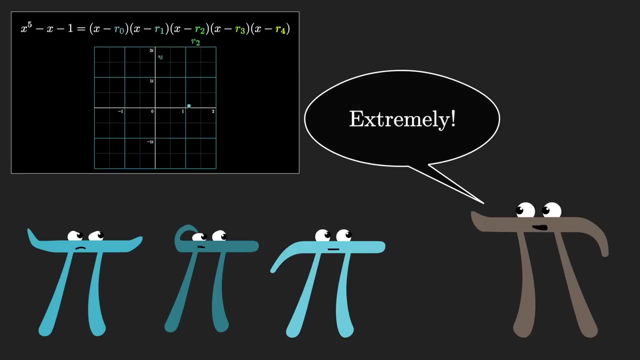 And so far you might be thinking: okay, this is intellectually playful enough, but is any of this actually useful? One of the earliest applications of group theory came when mathematicians realized that the structure of these permutation groups tells us something about solutions to polynomial equations. 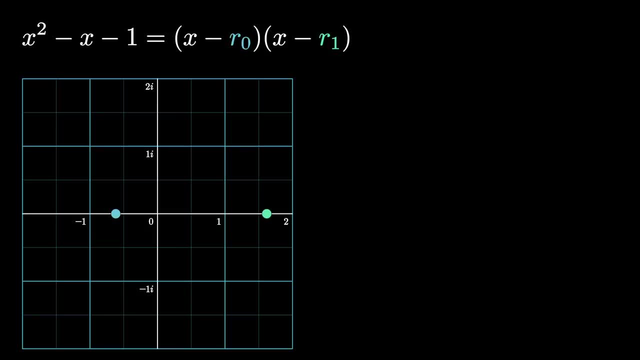 You know how, in order to find the two roots of a quadratic equation, everyone learns a certain formula in school. Slightly lesser known is the fact that there's also a cubic formula, one that involves nesting cube roots with square roots in a larger expression. 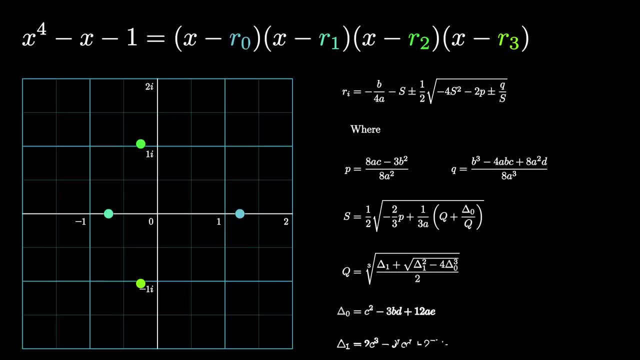 There's even a quartic formula for a degree-four polynomial, which is an absolute mess. It's almost impossible to write without factoring things out, And for the longest time mathematicians' struggled to find a formula to solve degree-five polynomials. Maybe there's one, but it's. 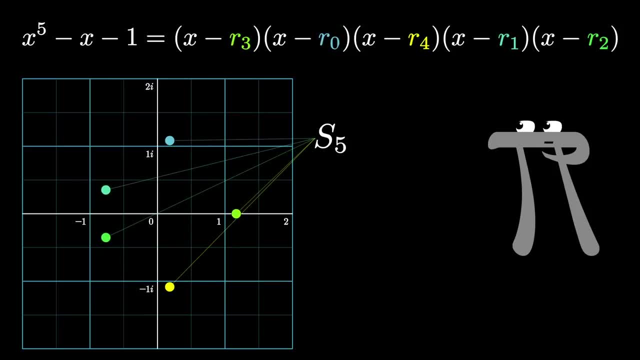 just super complicated. It turns out, though, if you think about the group which permutes the roots of such a polynomial, there's something about the nature of this group that reveals no quintic formula can exist. For example, the five roots of the polynomial you see on screen now have definite values. 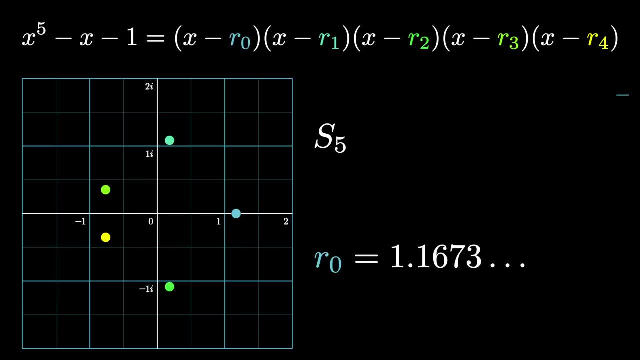 You could write out decimal approximations, but what you can never do is write those exact values by starting with the coefficients of the polynomial, And then you can never write those exact values by starting with the coefficients of the polynomial, And then you can never write those exact values by starting with the coefficients of the polynomial. 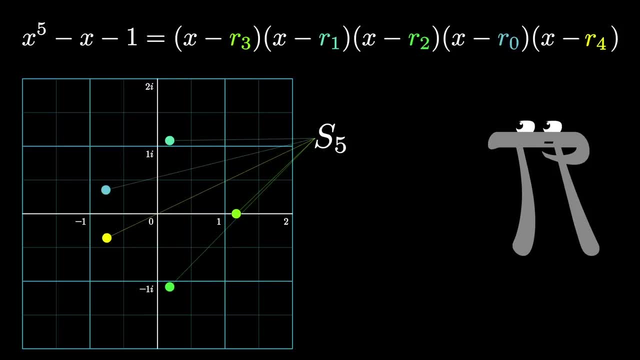 It turns out, though, if you think about the group which permutes the roots of such a polynomial, there's something about the nature of this group that reveals no quintic formula can exist. For example, the five roots of the polynomial you see on screen now, they have definite values. You could write out decimal approximations. But what you can never do is write those exact values by starting with the coefficients of the polynomial. And using only the four basic operations of arithmetic together with radicals, no matter how many times you nest them. And that impossibility has everything to do with the inner structure of the permutation group S5. 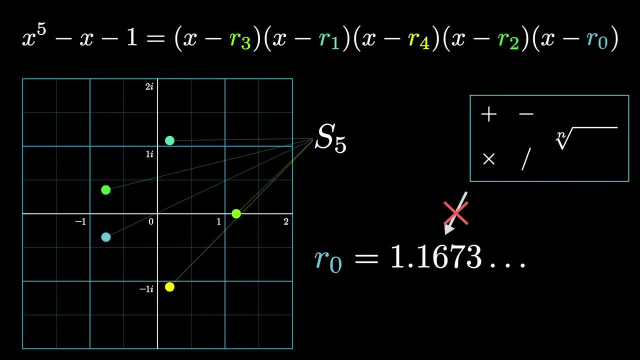 A theme in math through the last two centuries has been that the nature of symmetry in and of itself can show us all sorts of non-obvious facts about the other objects that we study. 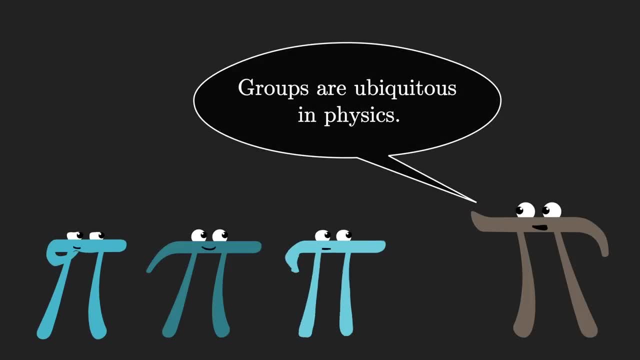 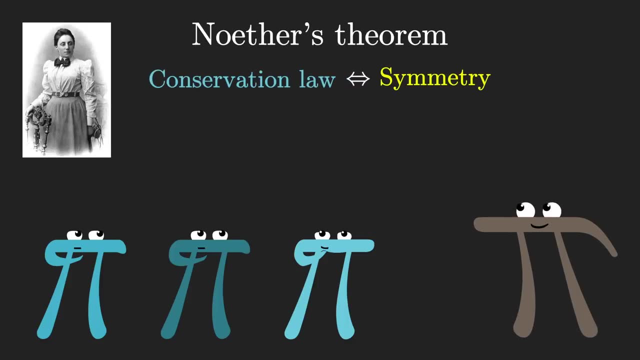 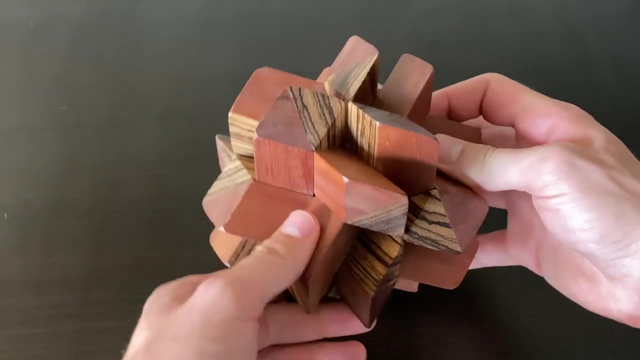 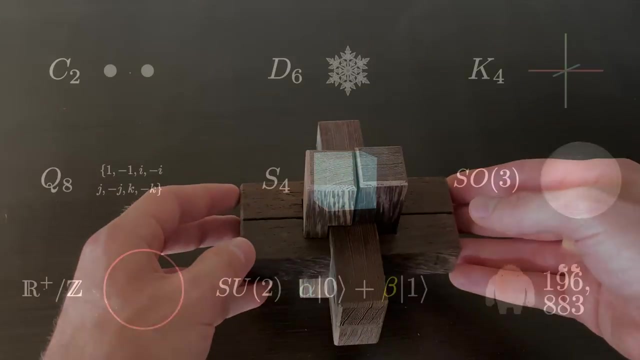 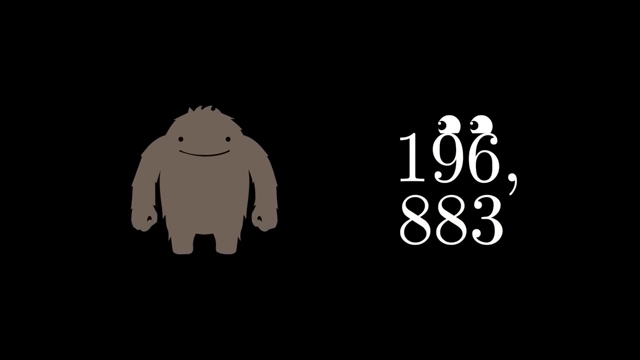 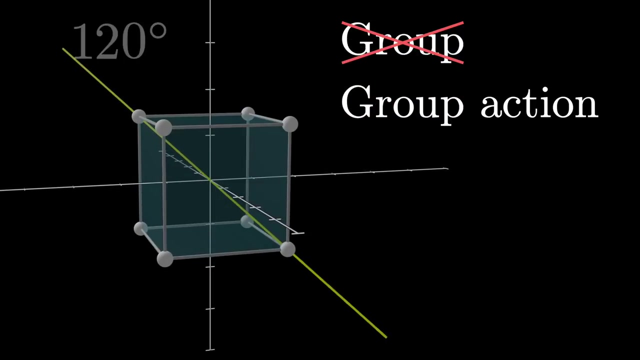 To give just a hint of the many, many ways that this applies to physics, there's a beautiful fact known as Noether's theorem saying that every conservation law corresponds to some kind of symmetry, a certain group. So all those fundamental laws like conservation of momentum and conservation of energy each correspond to a group. More specifically, the actions we should be able to apply to a setup such that the laws of physics don't change. All of this is to say that groups really are fundamental. And the one thing I want you to recognize right now is that they are one of the most natural things that you could study. What could be more universal than symmetry? So you might think that the patterns among groups themselves would somehow be very beautiful and symmetric. The monster, however, tells a different story. Before we get to the monster, though, at this point some mathematicians might complain that what I've described so far are not groups exactly, but group actions, and that groups are something slightly more abstract. 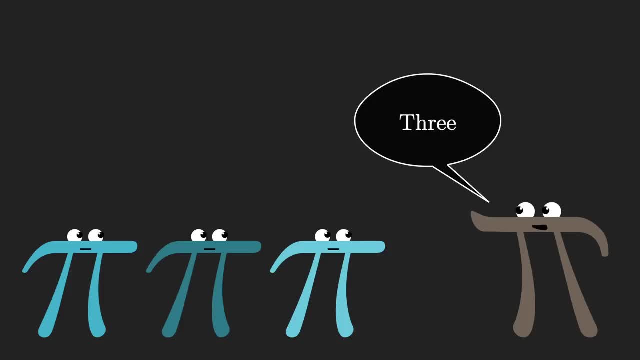 By way of analogy, if I mention the number three, you probably don't think about a specific triplet 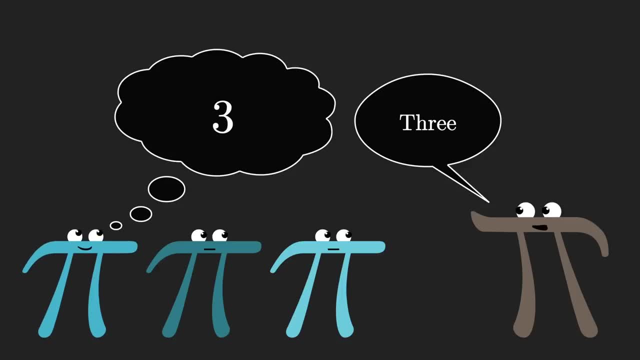 of things. You probably think about three as an object in and of itself. 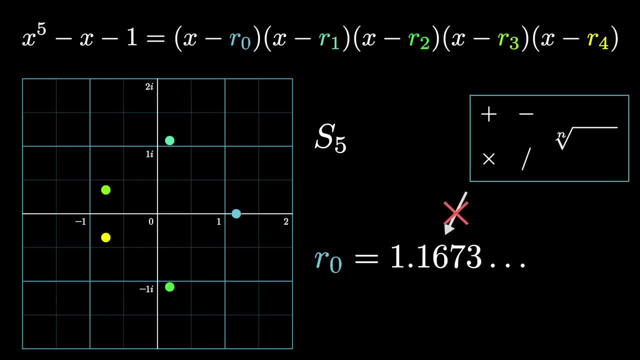 and using only the four basic operations of arithmetic, together with radicals, no matter how many times you nest them. and that impossibility has everything to do with the inner structure of the permutation group S5.. A theme in math through the last two centuries has been that the nature of symmetry in and of itself. 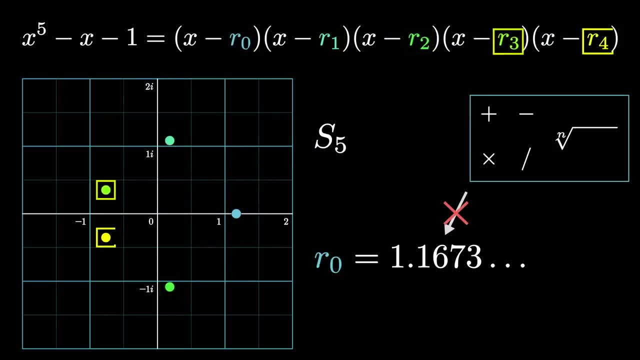 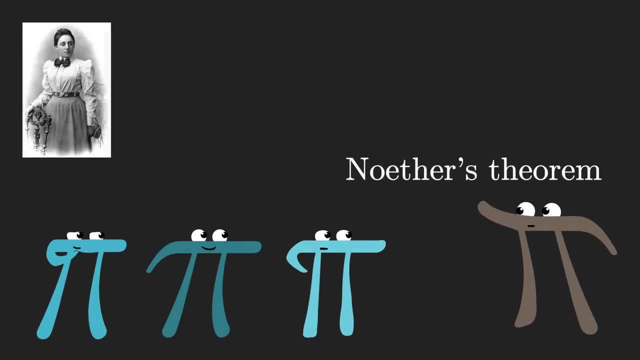 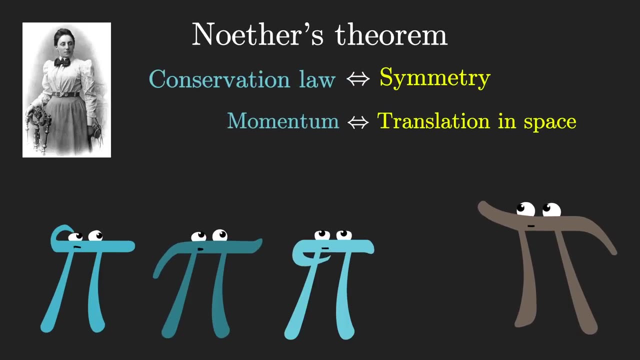 can show us all sorts of non-obvious facts about the other objects that we study. To give just a hint of the many, many ways that this applies to physics, there's a beautiful fact known as Noether's theorem, saying that every conservation law corresponds to some kind of symmetry, a certain group, So all those fundamental laws like 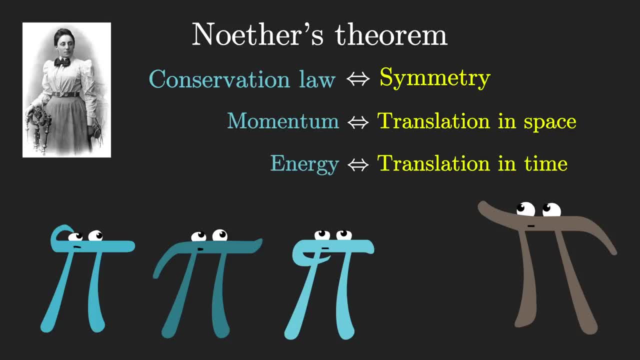 conservation of momentum and conservation of energy each correspond to a group. More specifically, the actions we should be able to apply to a setup such that the laws of physics don't change. All of this is to say that groups really are fundamental, and the one thing I want you to. 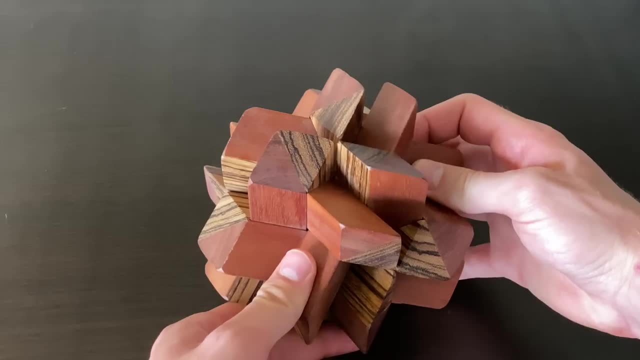 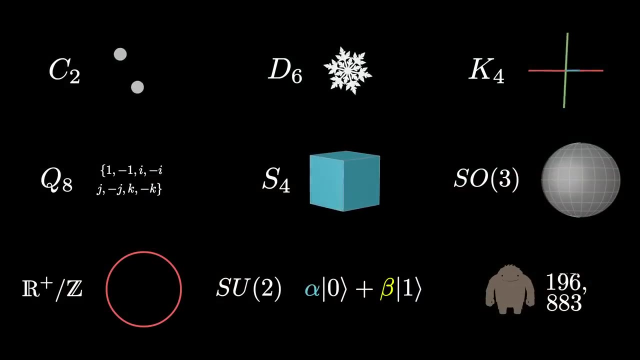 recognize right now is that they are one of the most natural things that you could study. What could be more universal? What could be more universal than symmetry? So you might think that the patterns among groups themselves would somehow be very beautiful and symmetric. The monster, however, tells a different story. Before we get to the monster, though. 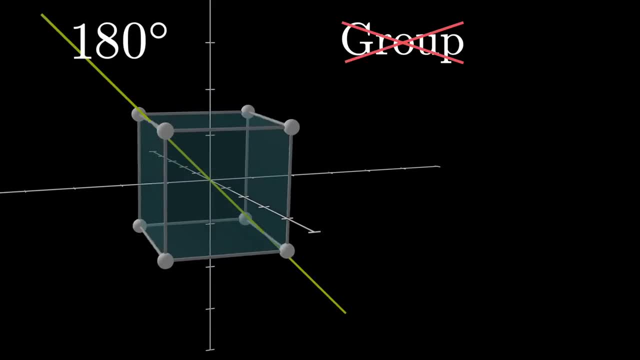 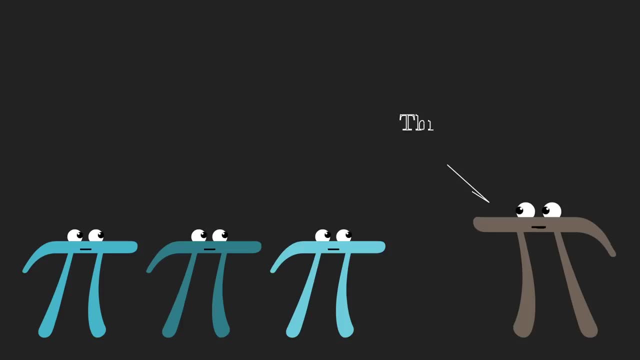 at this point, some mathematicians might complain that what I've described so far are not groups exactly, but group actions, and that groups are something slightly more abstract. By way of analogy, if I mention the number three, you probably don't think about a specific triplet. 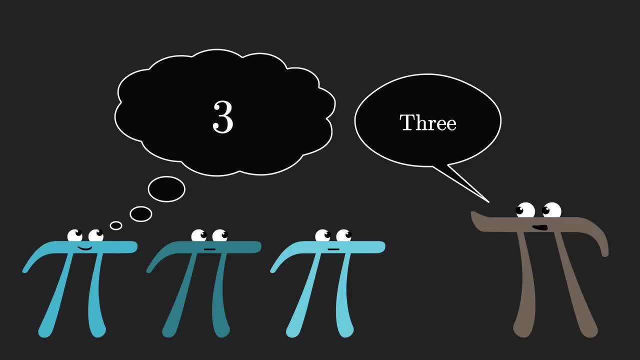 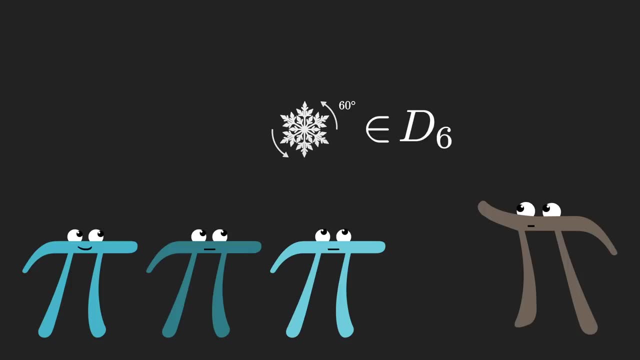 of things. You probably think about three as an object in and of itself, An abstraction, maybe represented with a symbol. In much the same way, when mathematicians discuss the elements of a group, they don't necessarily think about specific actions on specific objects. They might think of these elements as a kind of thing in and of itself. 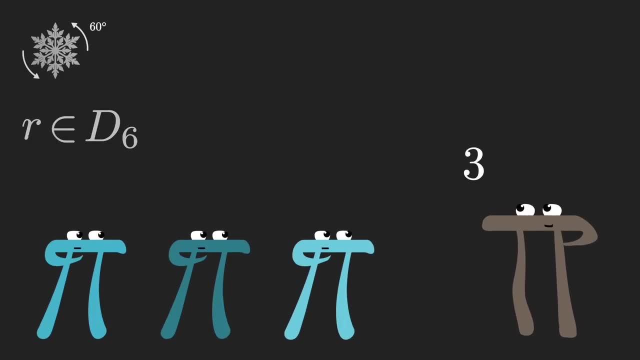 maybe represented with a symbol For something like the number three. the abstract symbol does us very little good unless we define its relation with other numbers, for example the way it adds or multiplies with them. For each of these, you could think of a. 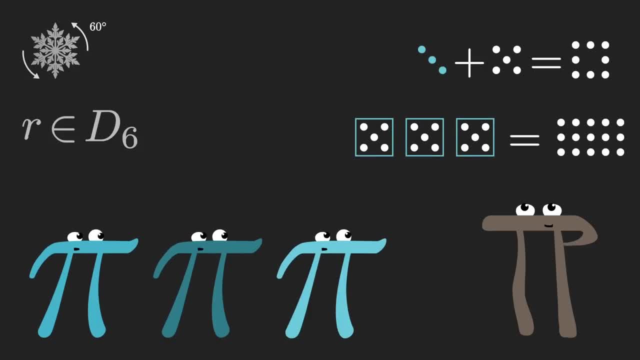 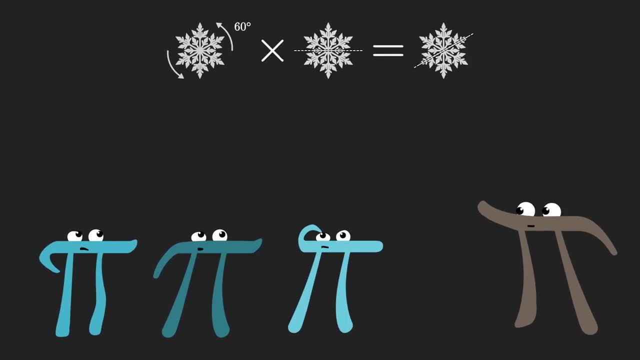 literal triplet of something. Again, most of us are comfortable- probably even more comfortable- using the symbols alone. Similarly, what makes a group a group are all of the ways that its elements combine with each other, And in the context of actions, this has a very vivid meaning. What we mean by combining is to 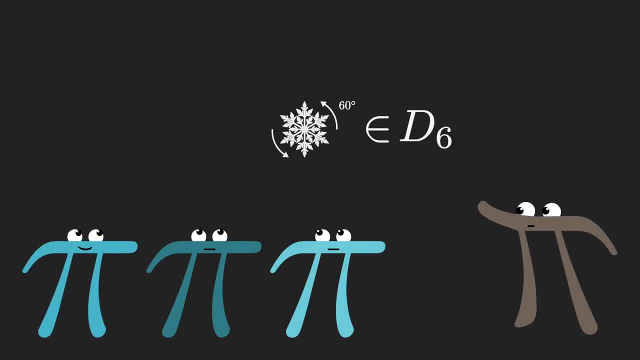 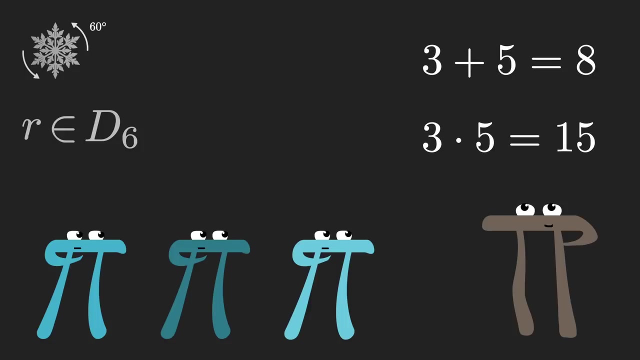 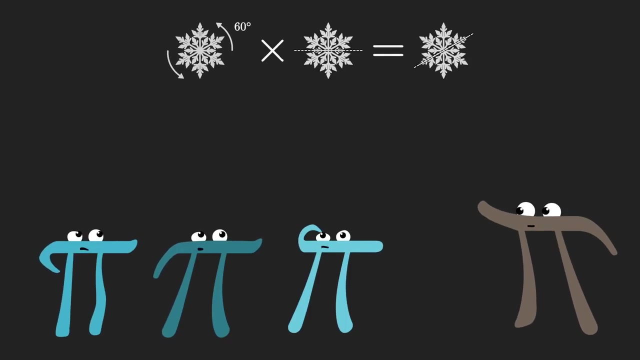 An abstraction may be represented with a symbol. In much the same way, when mathematicians discuss the elements of a group, they don't necessarily think about specific actions on specific objects. They might think of these elements as a kind of thing in and of itself, maybe represented with a symbol. For something like the number three, the abstract symbol does us very little good unless we define its relation with other numbers, for example the way that it adds or that it multiplies with them. For each of these, you could think of a literal triplet of something, but again, most of us are comfortable, probably even more comfortable, using the symbols alone. Similarly, what makes a group a group are all of the ways that its elements combine with each other. And in the context of actions, this has a very vivid meaning. What we mean by combining is to apply one action after the other, read from right to left. If you flip a snowflake about the x-axis, then rotate it 60 degrees counterclockwise, the overall action is the same as if you had flipped it about a diagonal line. If you flip a snowflake about the x-axis, then rotate it 60 degrees counterclockwise, the overall action is the same as if you had flipped it about a diagonal line. 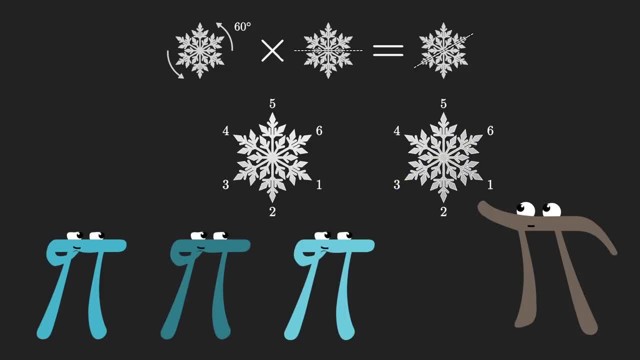 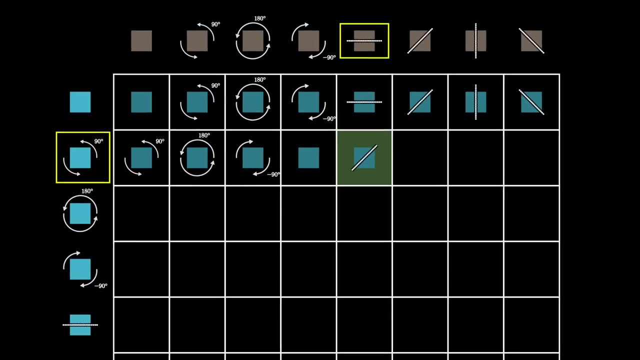 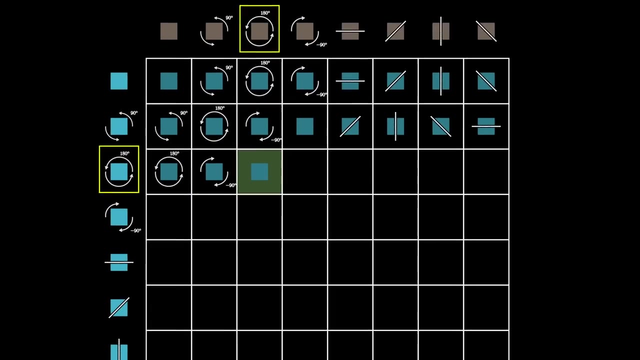 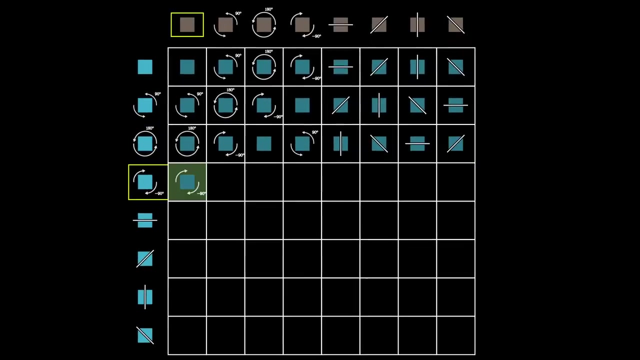 All possible ways that you can combine two elements of a group like this defines a kind of multiplication. That is what really gives a group its structure. Here, I'm drawing out the full 8x8 table of the symmetries of a square. If you apply an action from the top row and follow it by an action from the left column, it'll be the same as the action in the corresponding grid square. 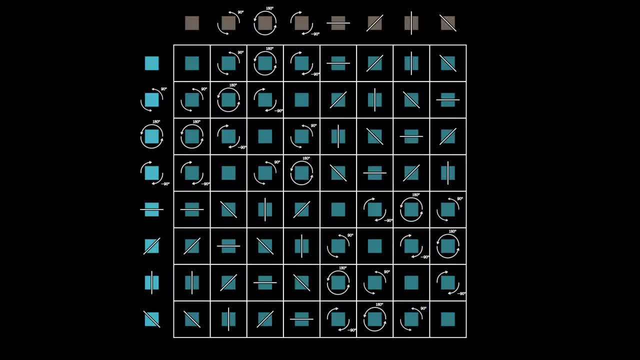 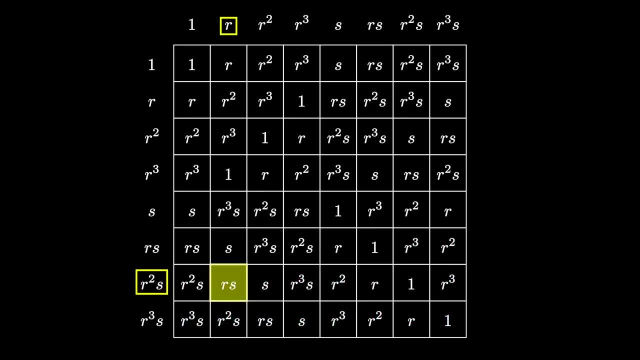 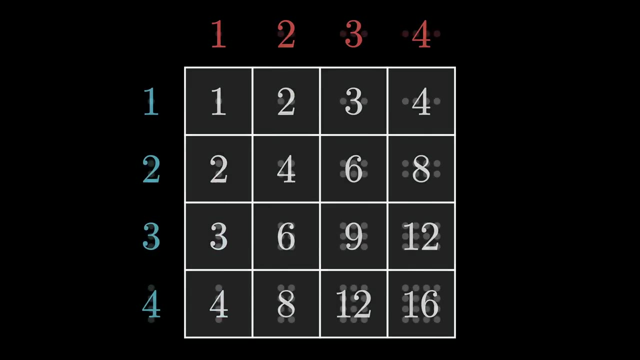 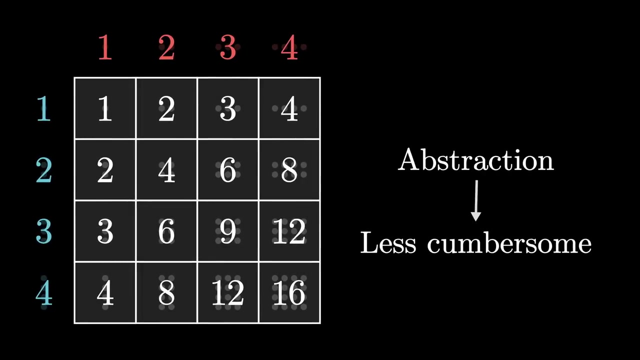 But if we replace each one of these symmetric actions with something purely symbolic, well, the multiplication table still captures the inner structure of the group, but now it's abstracted away from any specific object that it might act on, like a square or roots of a polynomial. This is entirely analogous to how the usual multiplication table is written symbolically, which abstracts away from the idea of literal counts. Literal counts, arguably, would make it much clearer what's going on. But if we replace each one of these symmetric actions with something symbolic, well, the multiplication table would make it much clearer what's going on. But since grade school, we all grow comfortable with the symbols. After all, they're less cumbersome, they free us to think about more complicated numbers, and they also free us to think about numbers in new and very different 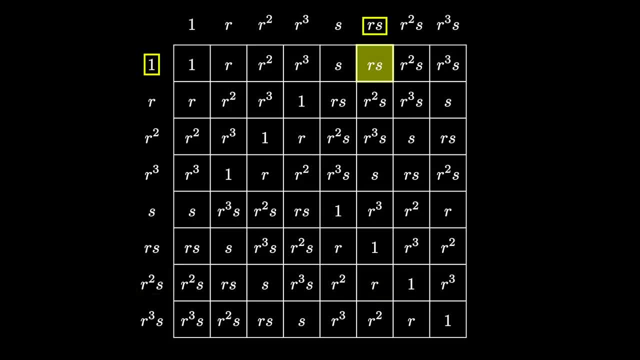 ways. All of this is true of groups as well, which are best understood as abstractions above the idea 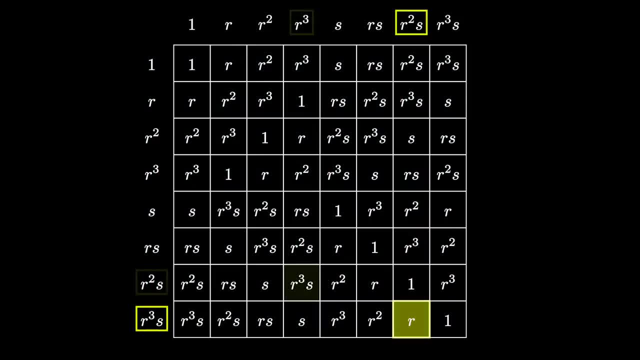 of symmetry actions. I'm emphasizing this for two reasons. One is that understanding what groups 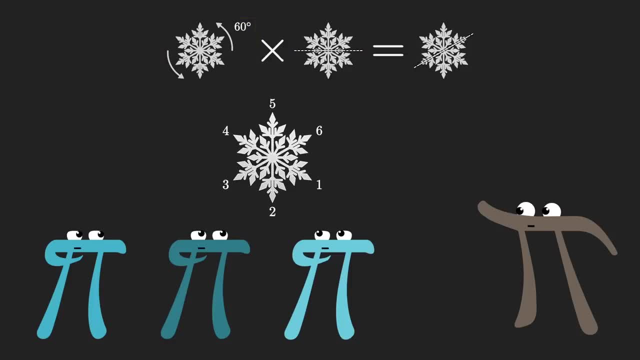 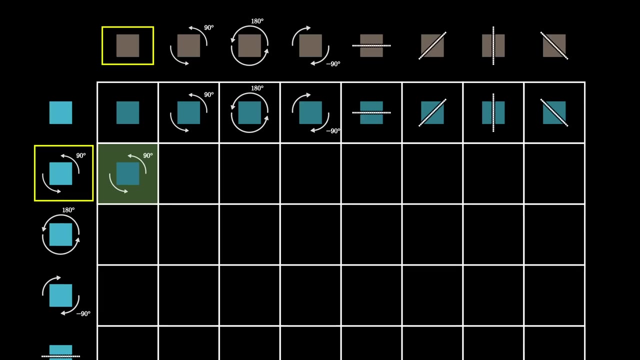 apply one action after the other. read from right to left. If you flip a snowflake about the x-axis, then rotate it 60 degrees counterclockwise. the overall action is the same as if you had flipped it about a diagonal line. 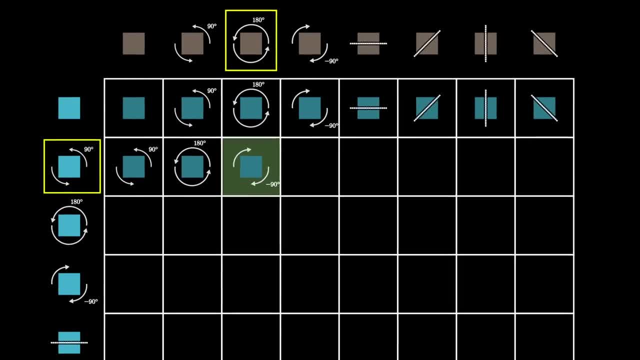 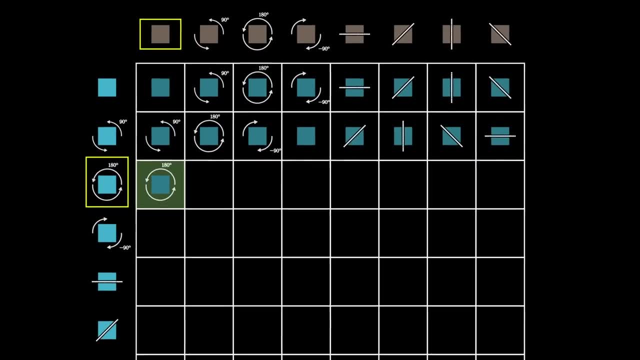 All possible ways that you can combine two elements of a group like this defines a kind of multiplication. That is what really gives a group its structure. Here I'm drawing out the full 8x8 table of the symmetries of a square. 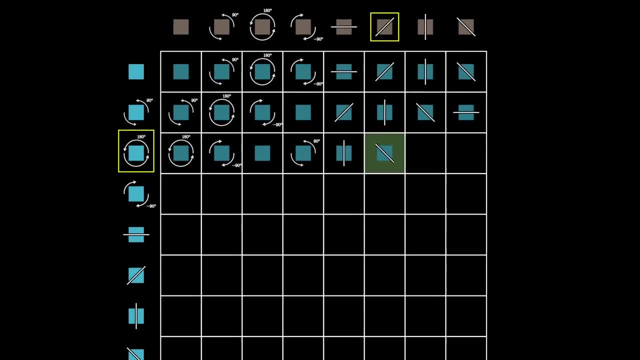 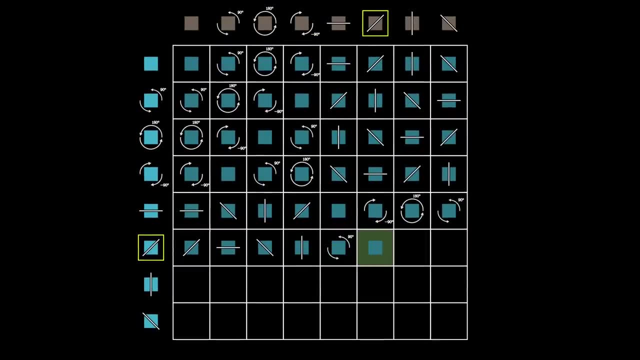 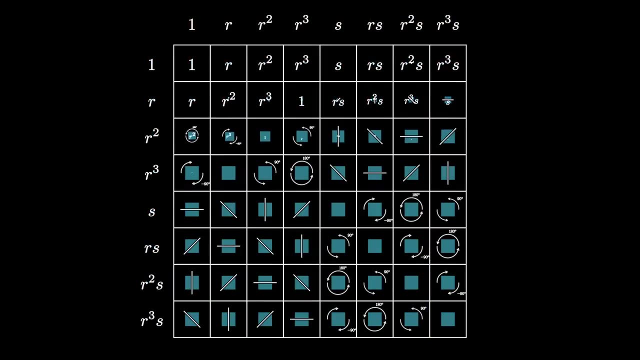 If you apply an action from the top row and follow it by an action from the left column, it'll be the same as the action in the corresponding grid square. But if we replace each one of these symmetric actions with something purely symbolic, well, the multiplication table still captures the inner structure of the group, but now it's. 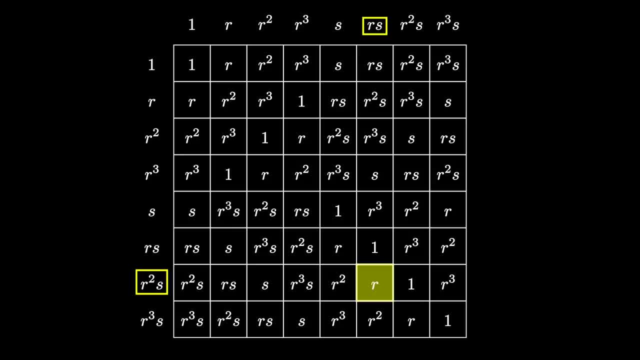 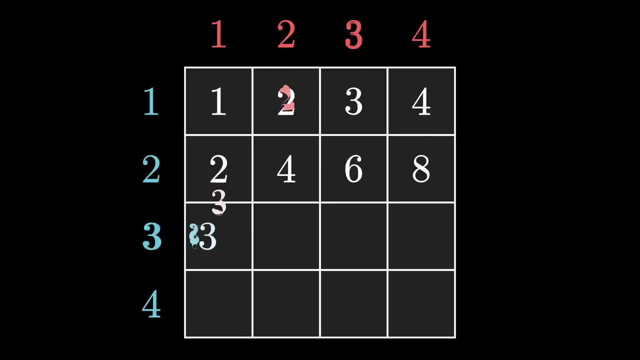 abstracted away from any specific object that it might act on, like a square or roots of a polynomial. This is entirely analogous to how the usual multiplication table is written symbolically, which abstracts away from the idea of literal counts. Literal counts arguably make it much clearer what's going on, but since grade school, 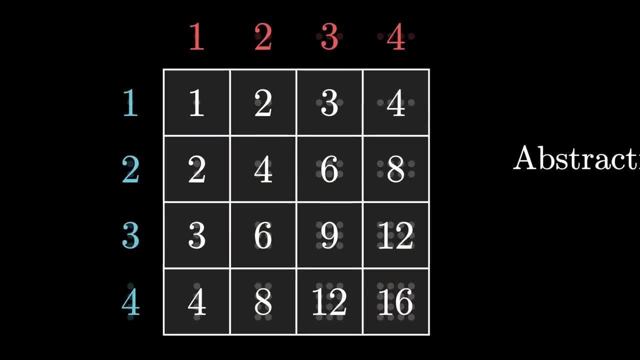 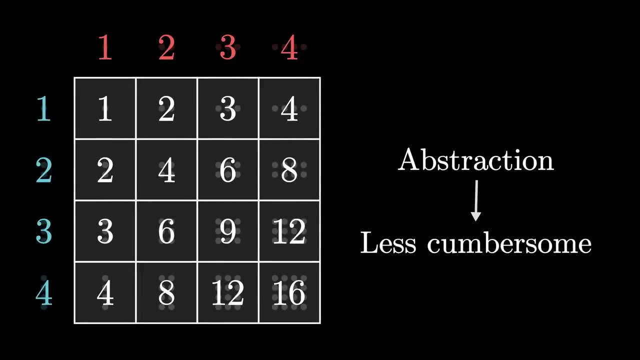 we all grow comfortable with the symbols. After all, they are less cumbersome, free us to think about more complicated numbers and free us to think about numbers in new and very different ways. All of this is true of groups as well, which are best understood as abstractions above. 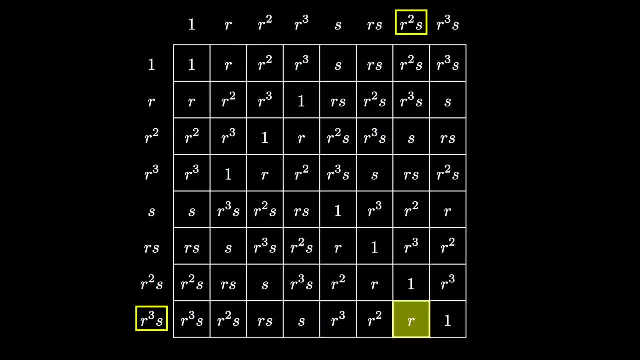 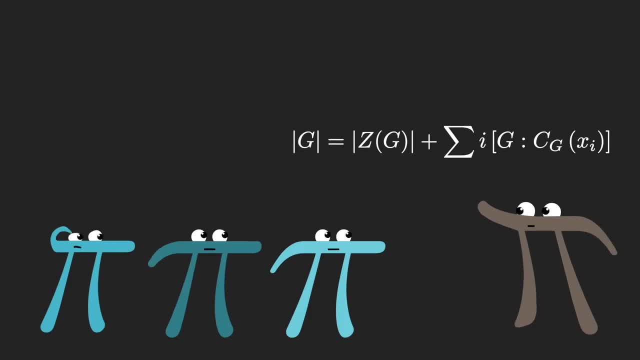 the idea of symmetry actions. I'm emphasizing this for two reasons. One is that understanding what groups really are gives a better appreciation for the monster, and the other is that many students learning about groups for the first time can find them frustratingly opaque. I know that. I 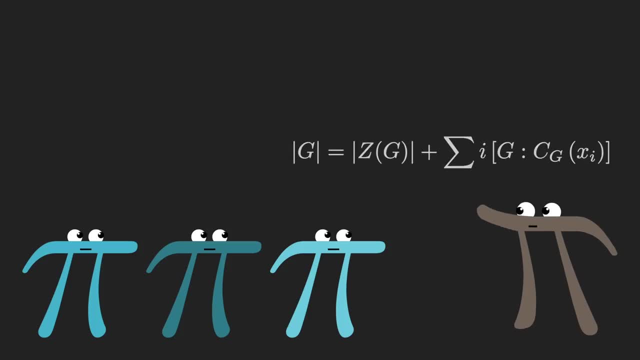 really are gives a better appreciation for the monster. And the other is that many students learning about groups for the first time can find them frustratingly difficult to understand. 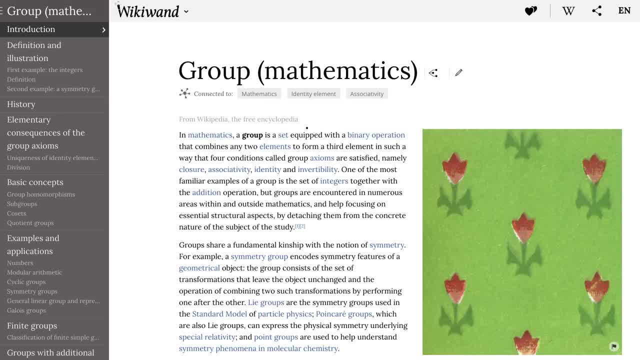 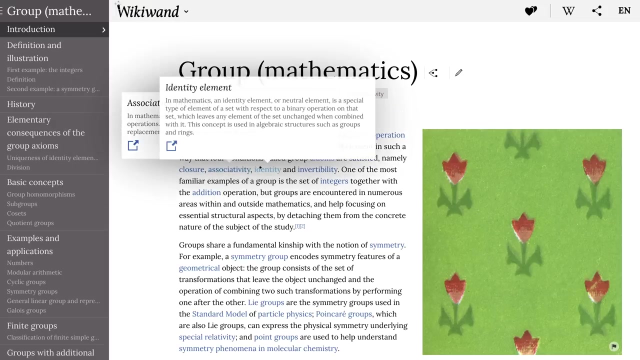 I know that I did. A typical course starts with this very formal and abstract definition, which is that a group is a set, in a collection of things, with a binary operation, a notion of multiplication between those things, such that this multiplication satisfies four special rules, or axioms. And all of this can feel, well, kind of random, especially when it isn't made clear that all of these axioms arise from the things that must obviously be true when you're thinking about actions. And that's exactly what I'm trying to do here. I'm trying to make sure that all of these 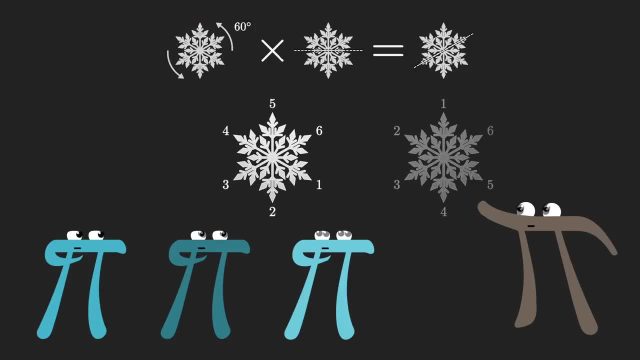 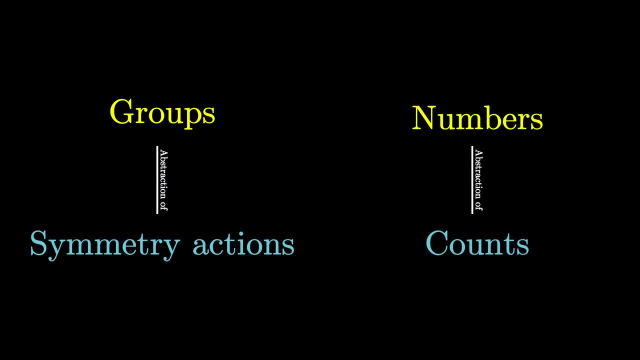 are abstractions and composing them. To any students among you with such a course in the future, I would say if you appreciate that the relationship groups have with symmetric actions is analogous to the relationship numbers have with counts, it can help to make the course a lot more 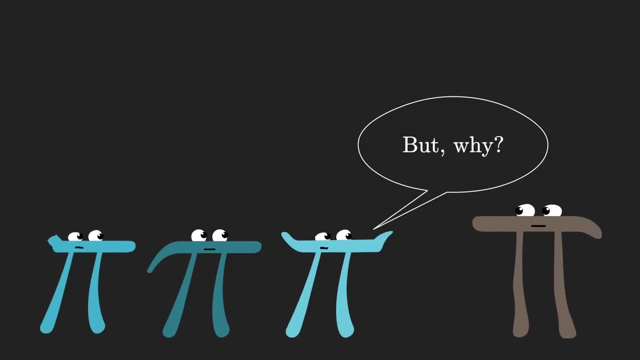 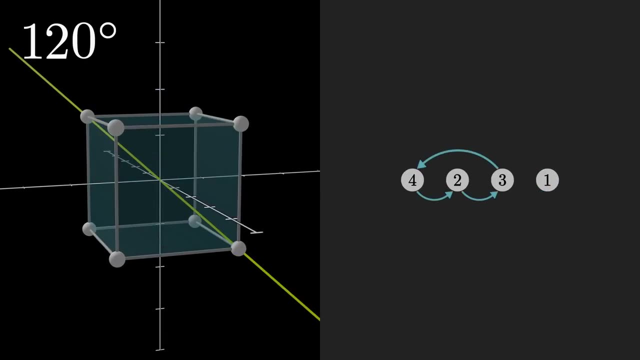 grounded. An example might help to see why this kind of abstraction is desirable. Consider the symmetries of a cube and the permutation group of four objects. At first, these groups feel very different. You might think of the one on the left as acting on eight corners, 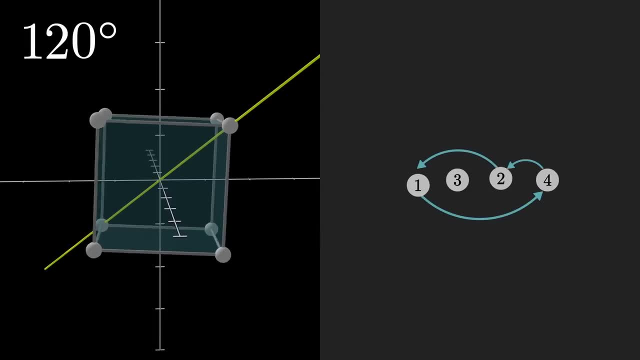 in a way that preserves the distance and orientation structure among them. But on the 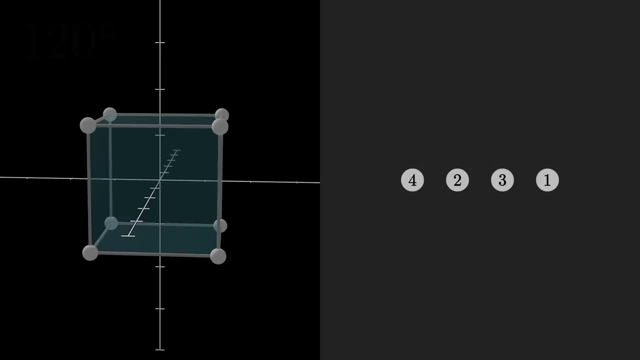 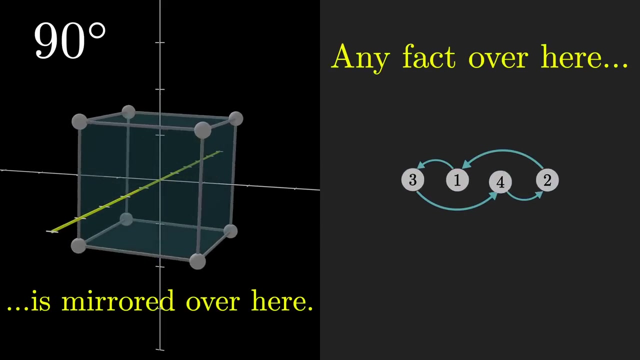 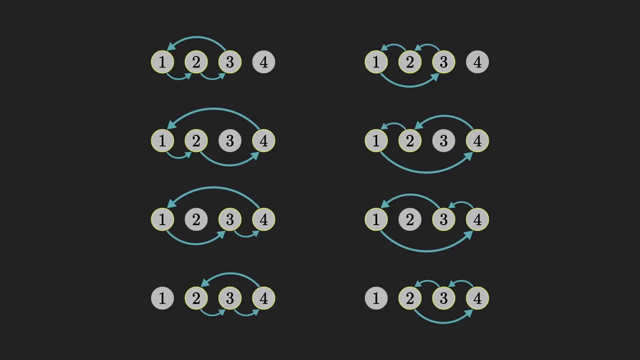 right, we have a completely unconstrained set of actions on a much smaller set of points. As it happens, though, these two groups are really the same, in the sense that their multiplication tables will look identical. Anything that you can say about one group will be true of the other. For example, there are eight distinct permutations where applying 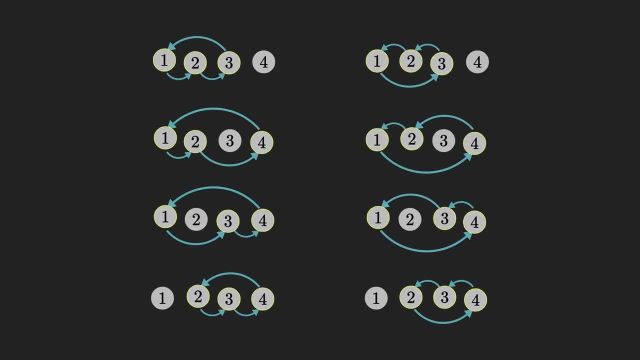 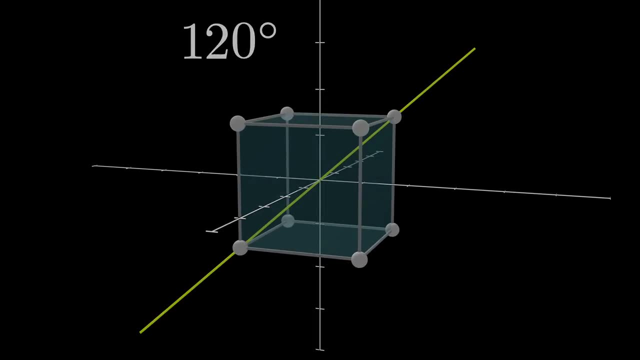 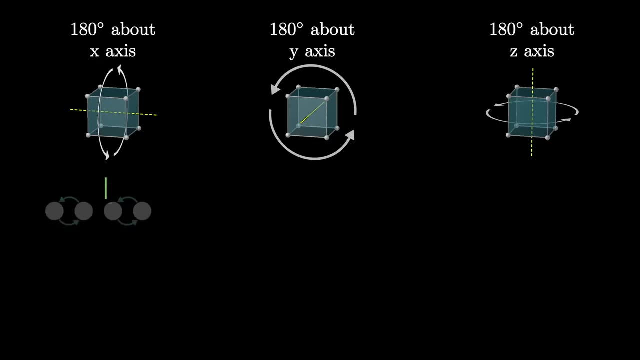 are the ones that cycle three different elements together. There are also eight rotations of the cube that have this property, the various 120 and 240 degree rotations about each diagonal. This is no coincidence. The way to phrase this more precisely is to say there is a one-to-one mapping between rotations of a cube and permutations of four elements which preserves 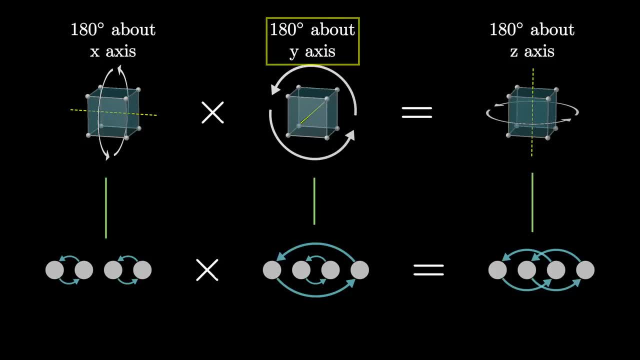 composition. For example, rotating 180 degrees about the y-axis followed by 180 degrees about the x-axis gives the same overall effect as rotating 180 degrees around the z-axis. 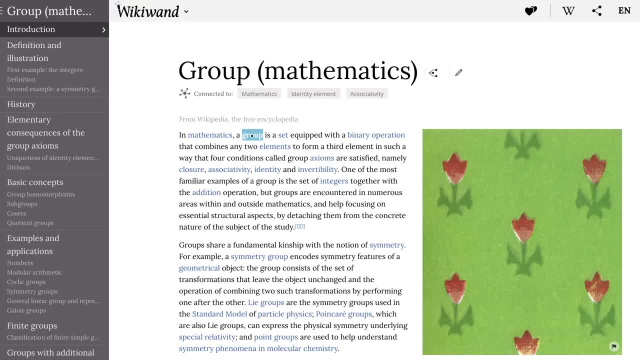 did. A typical course starts with this very formal and abstract definition, which is that a group is a set in a collection of things with a binary operation, a notion of multiplication between those things, such that this multiplication satisfies four special rules or axioms. 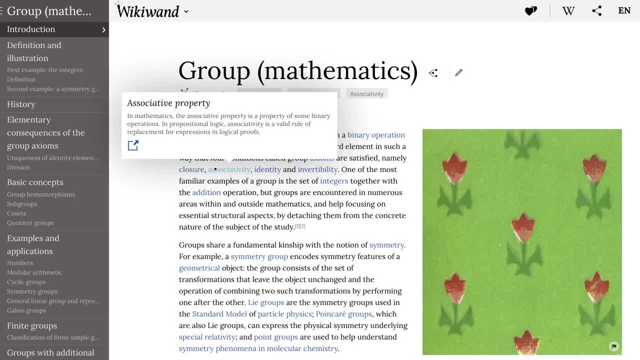 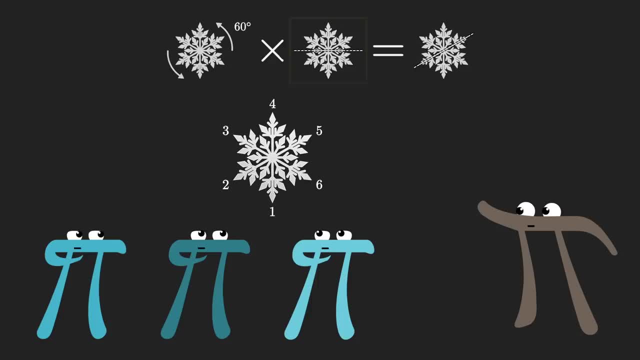 And all of this can feel well kind of random, especially when it isn't made clear that all of these axioms arise from the things. that must obviously be true when you're thinking about actions and composing them To any students among you with such a course in the future. 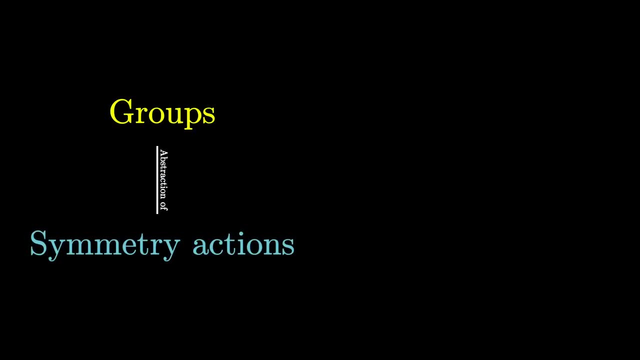 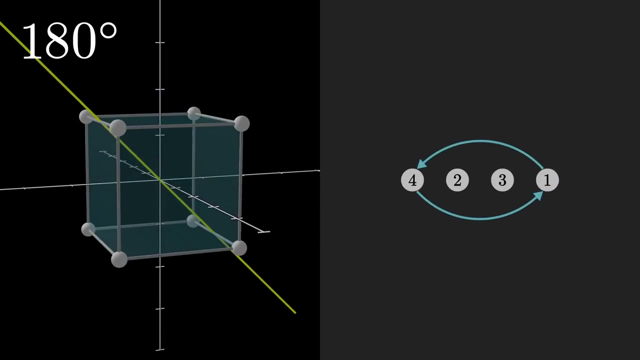 I would say if you appreciate that the relationship groups have with symmetric actions is analogous to the relationship numbers have with counts, it can help to make the course a lot more grounded. An example might help to see why this kind of abstraction is desirable. Consider the symmetries of a cube and the permutation group of four objects At first. 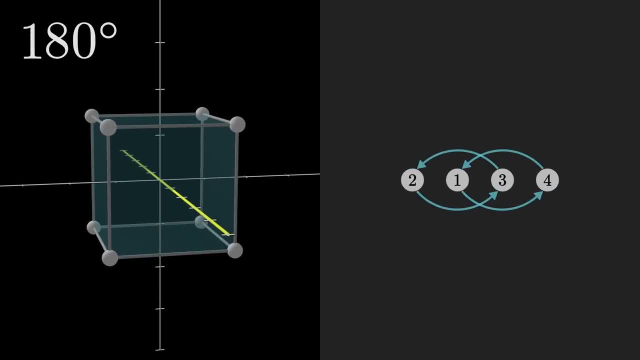 these groups feel very different. You might think of the one on the left as acting on eight corners in a way that preserves the distance and orientation structure among them, But on the right, we have a completely unconstrained set of actions on a much smaller set of points. 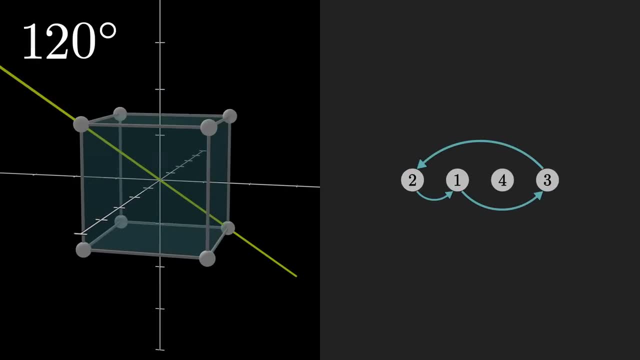 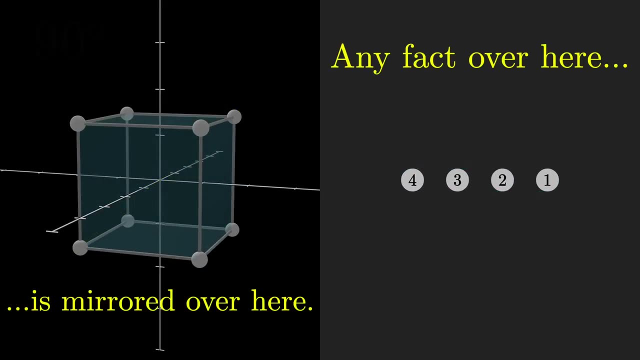 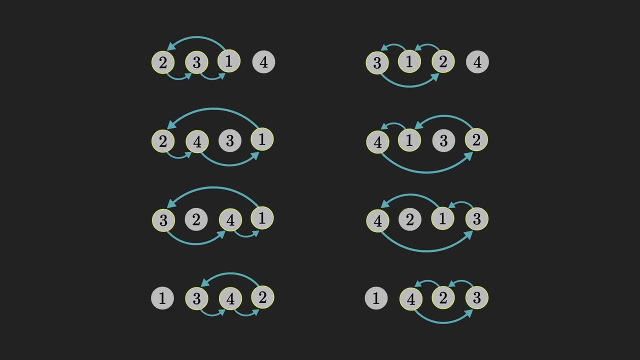 As it happens, though, these two groups are really the same in the sense that their multiplication tables will look identical. Anything that you can say about one group will be true of the other. For example, there are eight distinct permutations, where applying it three times in a row gets you back to where you started, not counting the identity These. 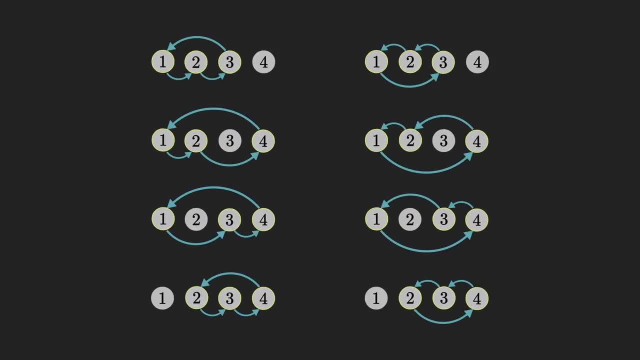 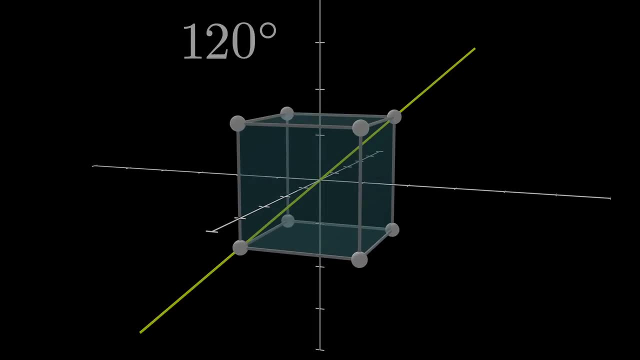 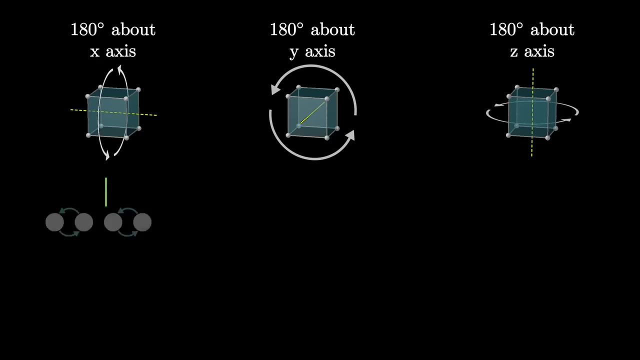 are the ones that cycle three different elements together. There are also eight rotations of the cube that have this property: the various 120 and 240 degree rotations about each diagonal. This is no coincidence. The way to phrase this more precisely is to say there is a one-to-one. 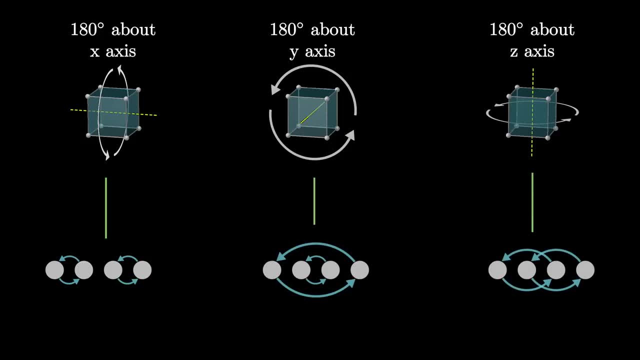 permutation between rotations of a cube and permutations of four elements, which preserves composition. For example, rotating 180 degrees about the y-axis followed by 180 degrees about the x-axis gives the same overall effect as rotating 180 degrees around the z-axis. 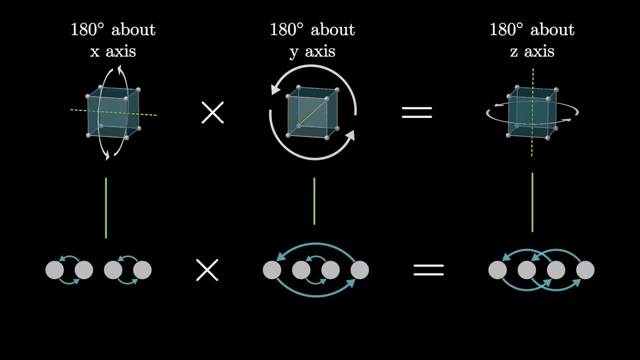 Remember, that's what we mean by a product of two actions And if you look at the corresponding permutations, under a certain one-to-one association, this product will still be true. Applying the two actions on the left gives the same overall effect as the one on the right When you have a correspondence where this remains true. 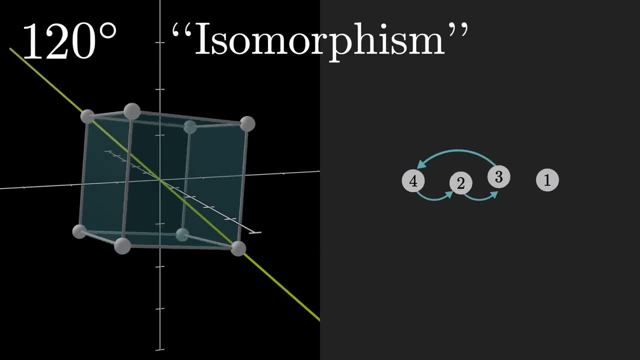 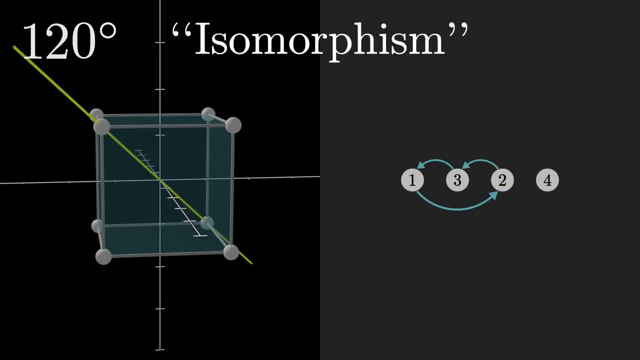 for all products. it's called an isomorphism, which is maybe the most important idea in group theory. This particular isomorphism between cube rotations and permutations of four objects is a bit subtle, but for the curious among you, you may enjoy taking a moment to think. 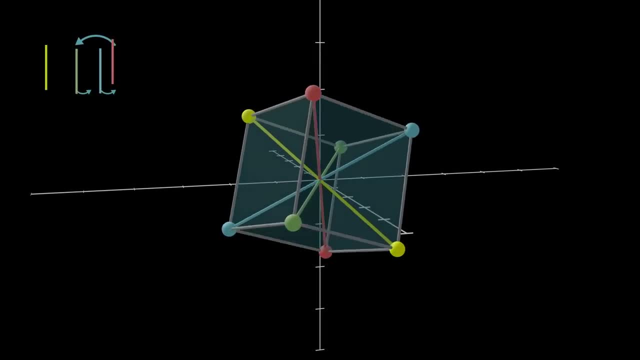 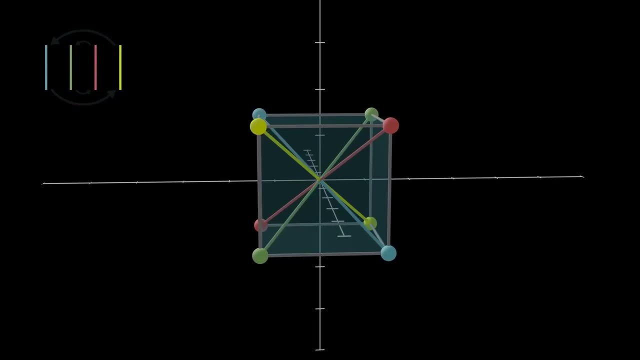 hard about how the rotations of a cube permute its four diagonals. In your mathematical life, you'll see more examples of a given group arising from seemingly unrelated situations, And as you do, you'll get a better sense for what group theory is all about. 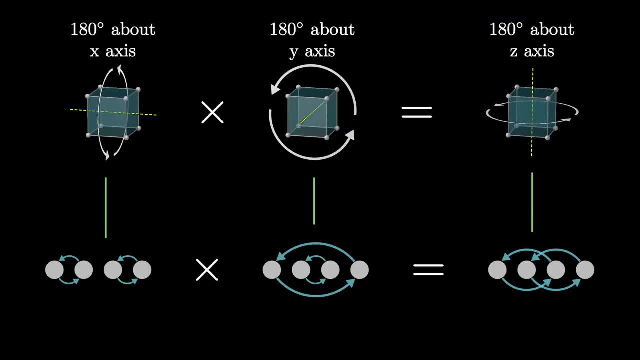 Remember, that's what we mean by a product of two actions. And if you look at the corresponding permutations under a certain one-to-one association, this product will still be true. Applying the two actions on the left gives the same overall effect as the one on the right. 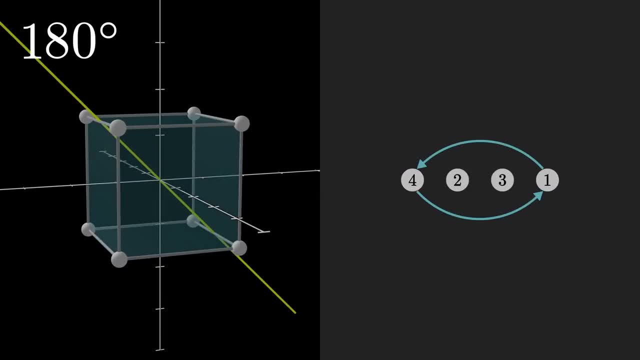 When you have a correspondence where this remains true for all products, it's called an isomorphism, which is maybe the most important idea in group theory. 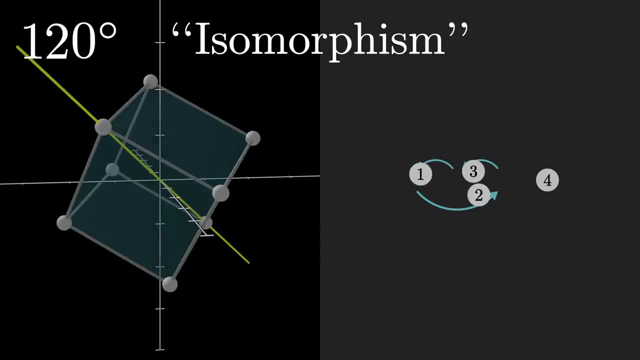 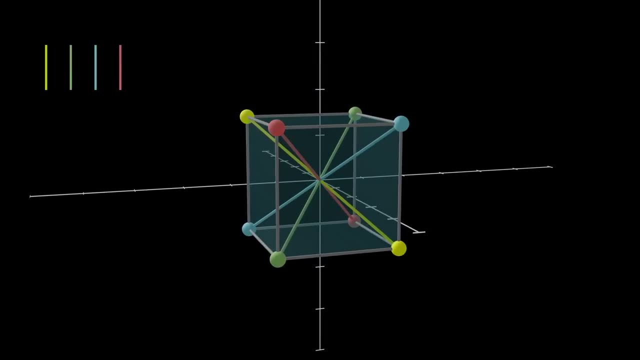 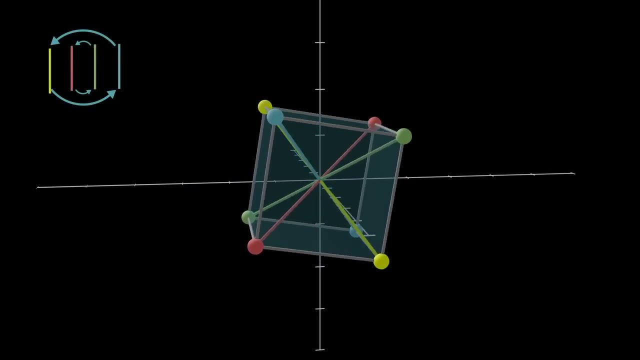 This particular isomorphism between cube rotations and permutations of four objects is a bit subtle, but for the curious among you, you may enjoy taking a moment to think hard about how the rotations of a cube permute its four diagonals. 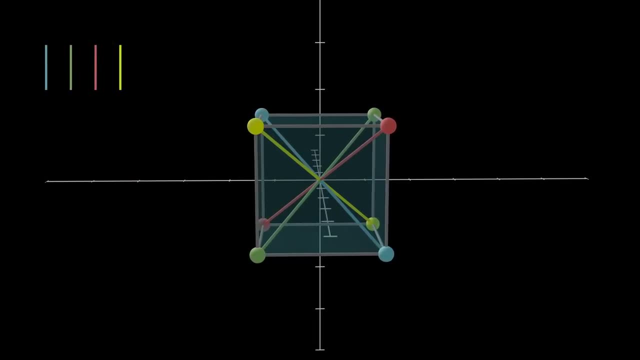 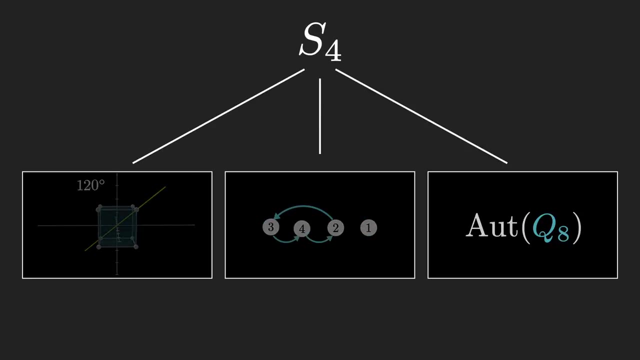 In your mathematical life, you'll see more examples of a given group arising from seemingly unrelated situations, and as you do, you'll get a better sense for what group theory is all about. Think about how a number like 3 is not really about a particular triplet of things. It's about all possible triplets of things. In the same way, a group 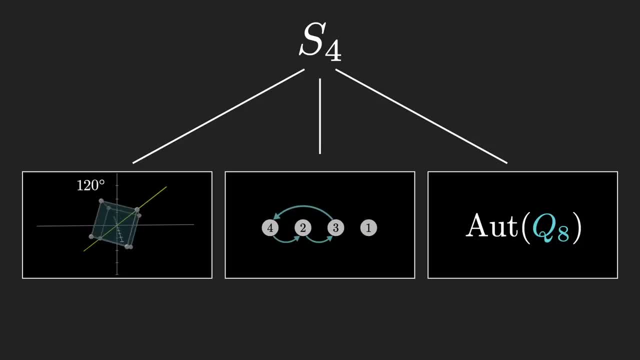 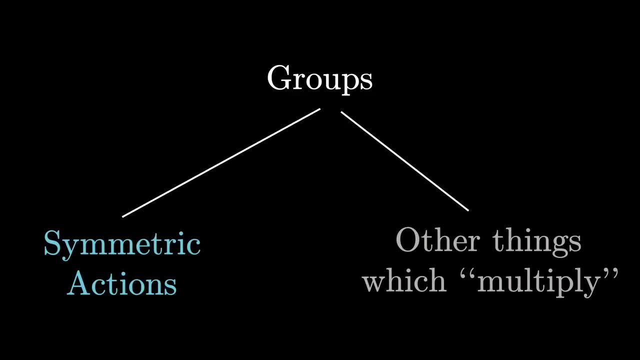 is not really about symmetries of a particular object. It's an abstract way that things even can be symmetric. There are even plenty of situations where groups come up in a way that does not feel like a set of symmetric actions at all, just as numbers can do a lot 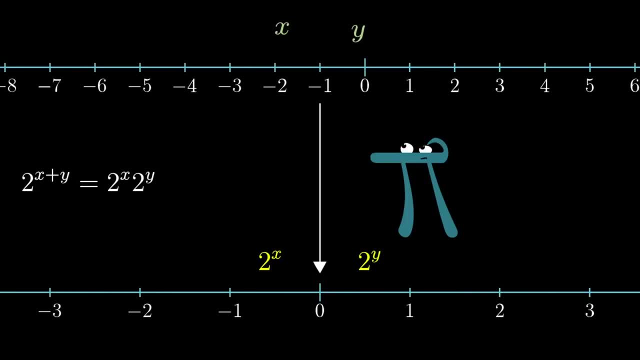 more than count. In fact, seeing the same group come up in different situations is a great way to reveal unexpected connections between distinct objects. That's a very common theme in modern math. 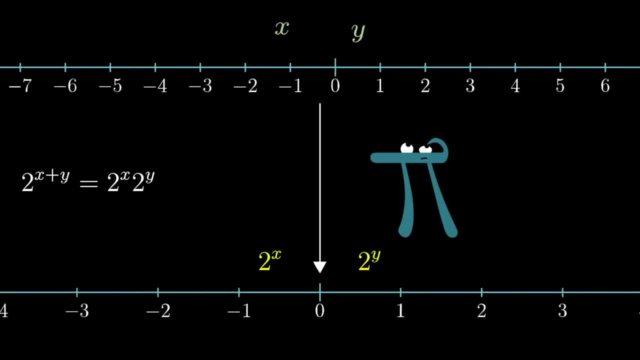 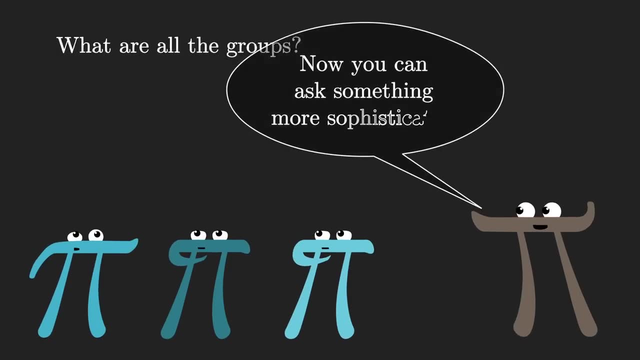 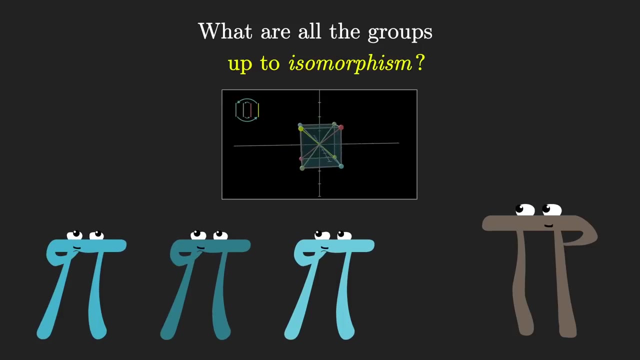 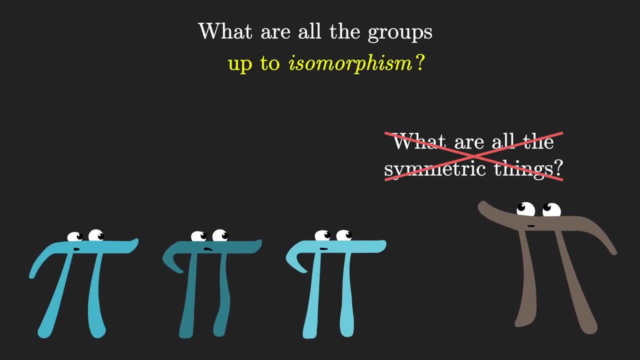 And once you understand this about groups, it leads you to a natural question, which will eventually lead to the monster. What are all the groups? But now you're in a position to ask that question in a more sophisticated way. What are all the groups up to isomorphism? Which is to say, we consider two groups to be the same if there's an isomorphism between them. This is asking something more fundamental than what are all the symmetric things. It's a way of asking what are all the ways that something can be symmetrical. 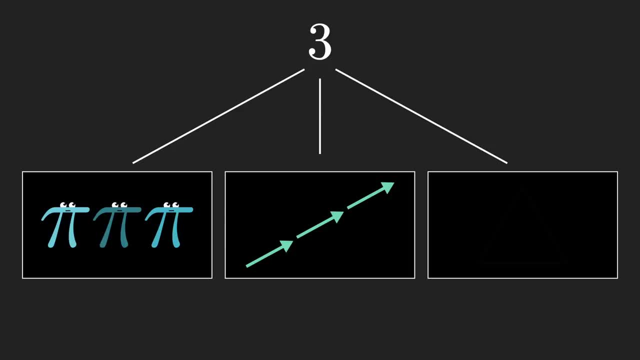 Think about how a number like 3 is not really about a particular triplet of things. It's about all possible triplets of things. In the same way, a group is not really about symmetries of a particular object. It's an abstract way that things even can be symmetric. There are even plenty of 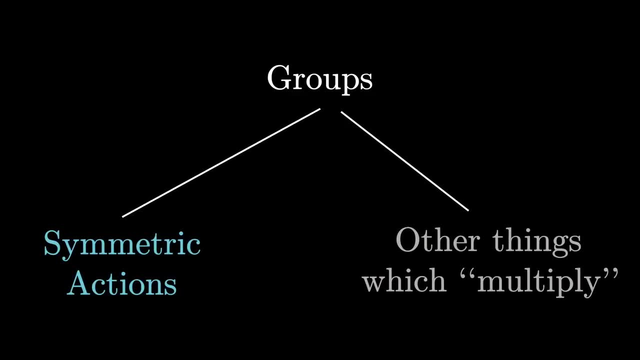 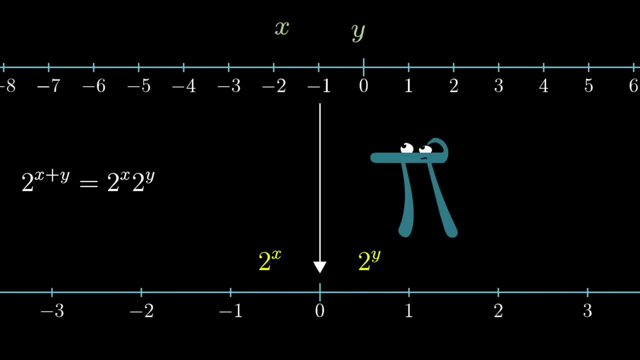 situations where groups come up in a way that does not feel like a set of symmetric actions at all, just as numbers can do a lot more than that. In fact, seeing the same group come up in different situations is a great way to reveal unexpected connections between distinct objects. That's a very common theme in modern math. 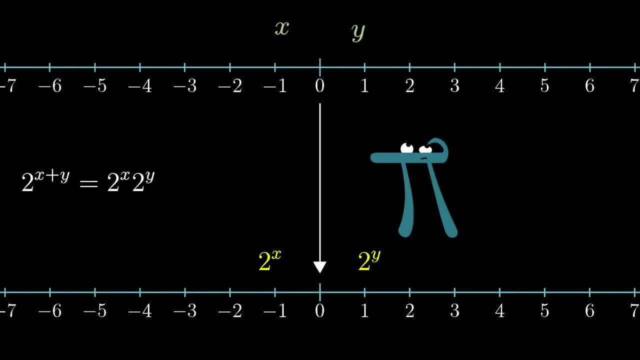 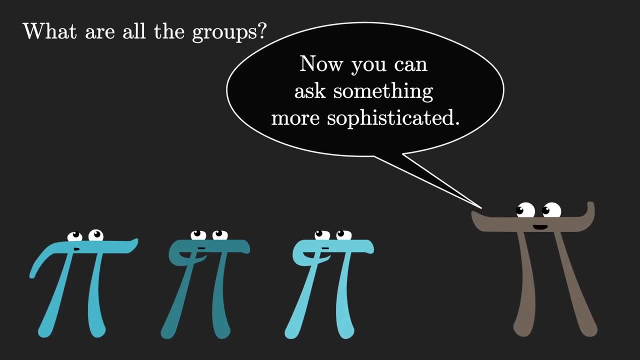 And once you understand this about groups, it leads you to a natural question which will eventually lead to the monster: What are all the groups? But now you're in a position to ask that question in a more sophisticated way: What are all the groups up to isomorphism, Which is to say we consider two groups to be the same if there's an isomorphism, Which is to say we consider two groups to be the same, if there's an isomorphism, Which is to say we consider two groups to be the same if there's an isomorphism between them. This is asking something more fundamental than what are all the symmetric things. It's a way of asking: what are all the ways that something can be symmetric? Is there some formula or procedure for producing them all, Some meta-pattern lying at the heart of symmetry itself? 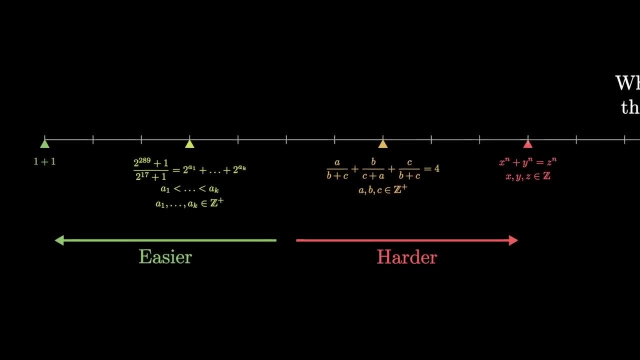 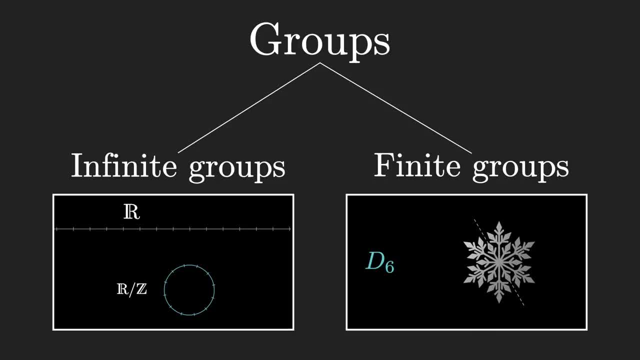 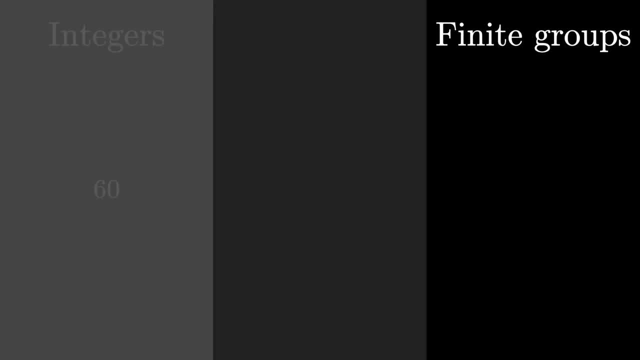 or the ones describing the symmetries of a line or a circle, and finite groups. To make up some hope of sanity, let's limit our view to finite groups In the same way that the numbers can be broken down into their prime factorization. 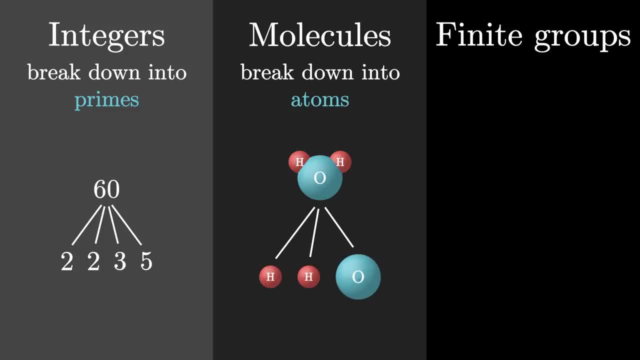 or molecules can be described based on atoms within them there's a certain way. finite groups can be broken down into a kind of composition of smaller groups. The ones which can't be broken down any further, analogous to prime numbers or atoms, are known as the simple groups. To give a hint. the otheruss snip großezendier is often seen as a period in the composition if there's a crimson in the dynamics of trasz week in the sievens where there is no dramatic shift between two North-South xtreme and two goin de S�es Busse. 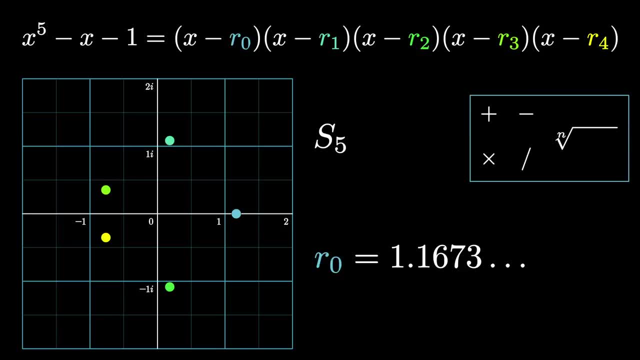 To give a hint, there are other fitting rhythmic PE aimings in there as well. for why this is useful: Remember how we said that group theory can be used to prove that there's no formula for a degree-five polynomial, the way there is for quadratic equations. 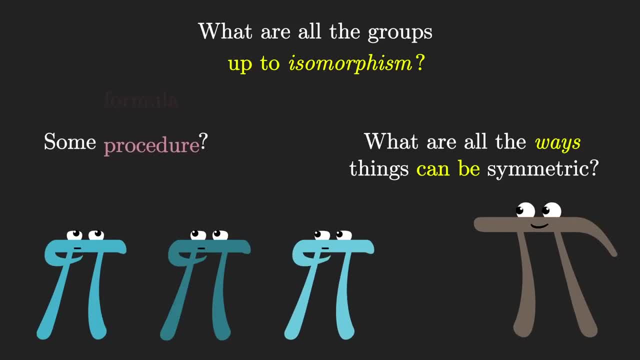 Is there some formula or procedure for producing them all, some meta-pattern lying at the heart 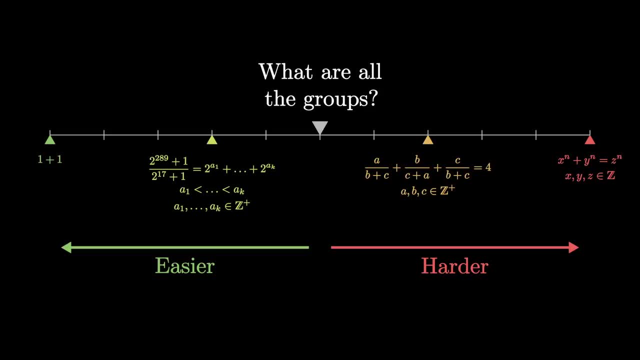 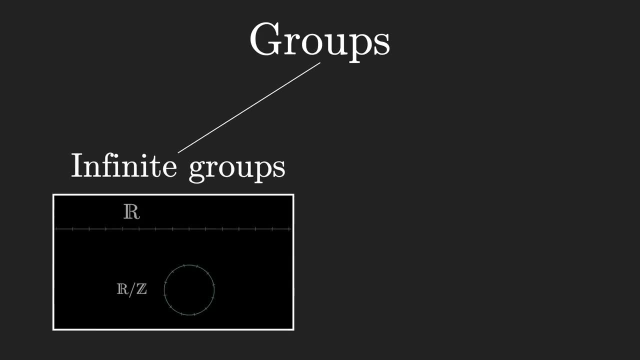 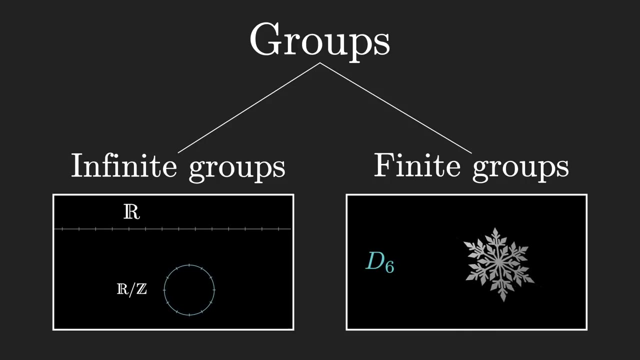 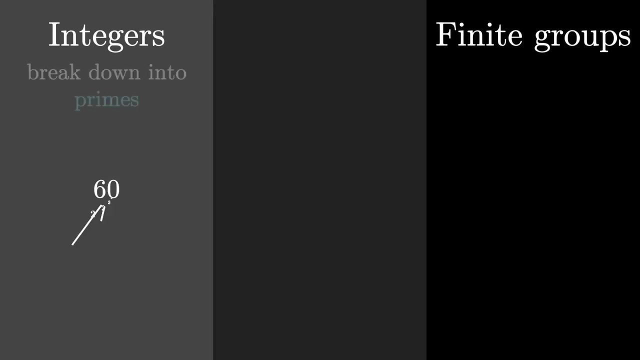 of symmetry itself? This question turns out to be hard. Exceedingly hard. For one thing, there's the division between infinite groups, for example the ones describing the symmetries of a line or a circle, and finite groups, like the ones we've looked at up to this point. To maintain some hope of sanity, let's limit our view to finite groups. In the same way that numbers can be broken down into different groups, numbers can be broken down into different types of groups, or molecules can be described based on the atoms within them, there's a certain way that finite groups can be broken down into a kind of composition of smaller groups. 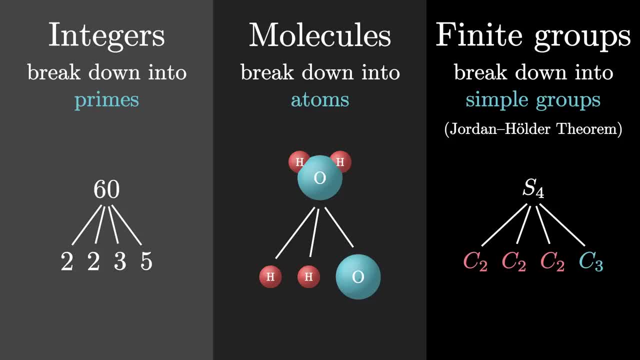 The ones which can't be broken down any further, analogous to prime numbers or atoms, 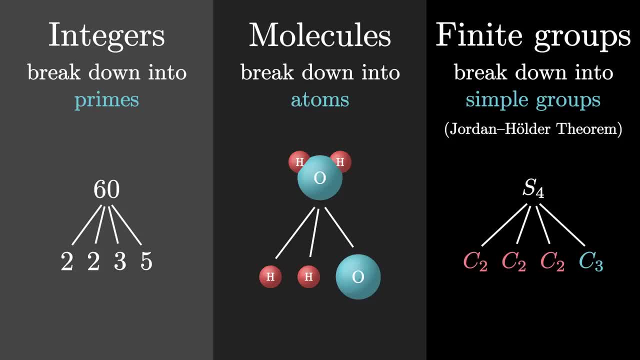 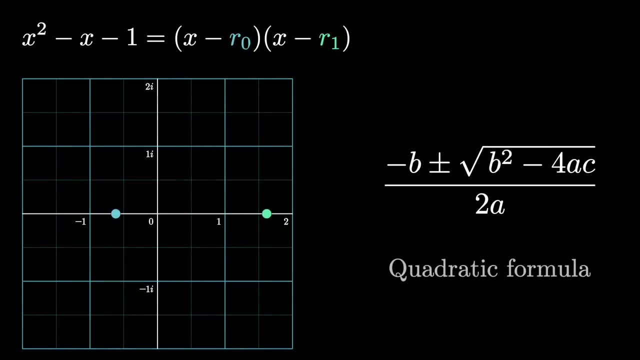 are known as the simple groups. To give a hint for why this is useful, remember how we said that group theory can be used to prove that there's no formula for a degree-five polynomial, the way there is for quadratic 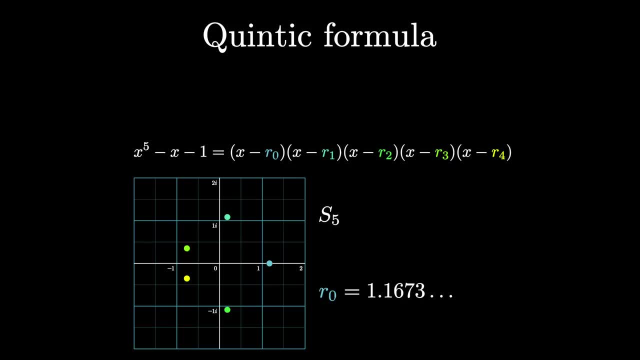 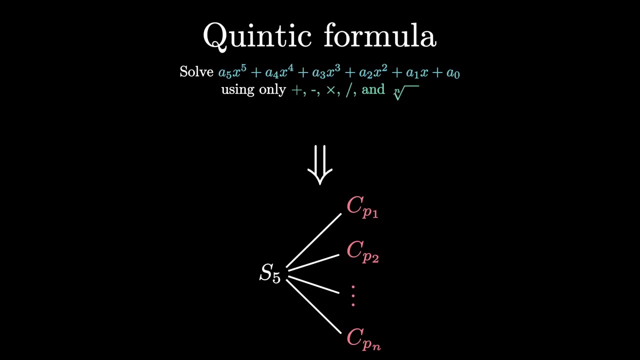 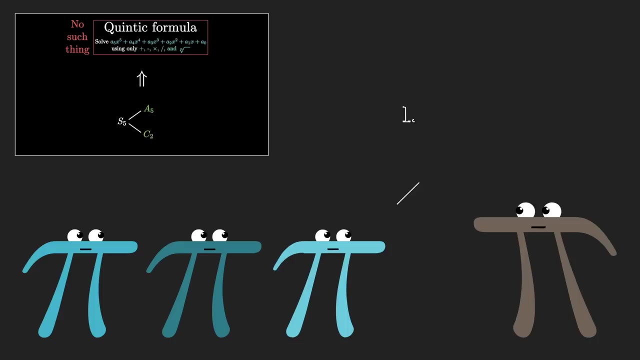 equations? Well, if you're wondering what that proof actually looks like, it's because it involves showing that if there were some kind of mythical quintic formula, something which uses only radicals and the basic arithmetic operations, it would imply that the permutation group on five elements decomposes into a special kind of simple group, known fancifully as the cyclic groups of prime order. But the actual way that this breaks down involves a different kind of simple group, a different kind of atom, one which polynomial solutions built from radicals would never allow. That is a super high-level description. 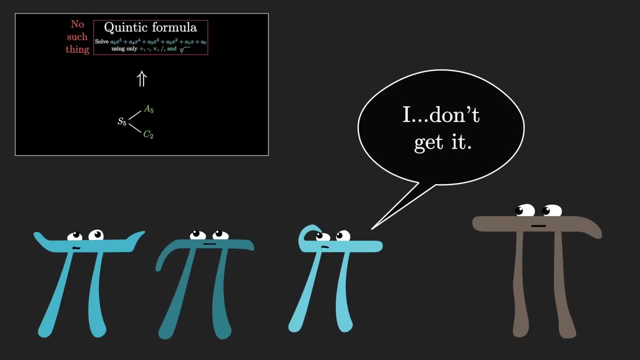 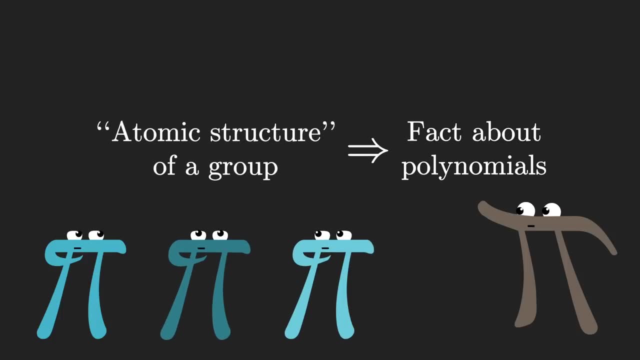 The point is that you have this really not-obvious fact about a different part of math whose solutions come from finding the atomic structure of a certain group. This is one of many different 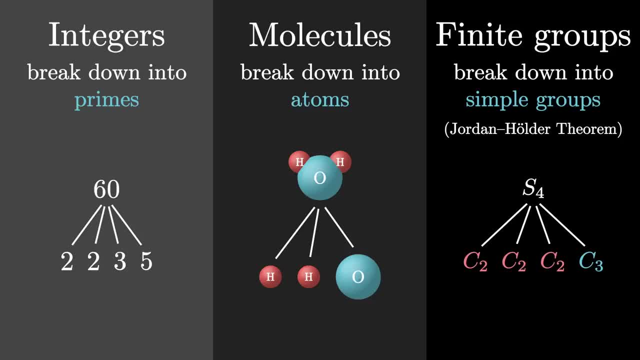 examples where understanding the nature of these simple groups, these atoms, actually matters outside of group theory. 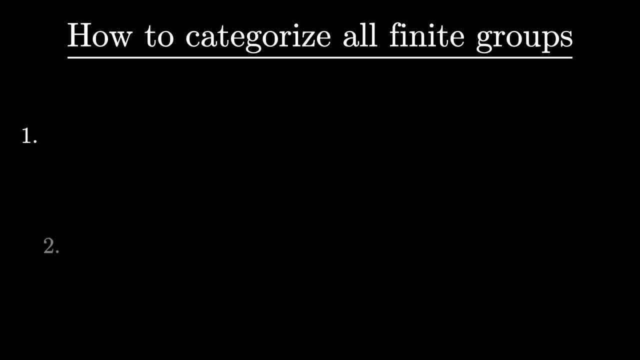 The task of categorizing all finite groups breaks down into two steps. One, find all the simple groups, and two, find all of the ways to combine them. The first question is finding the periodic table, and the second is a bit like doing all of chemistry thereafter. 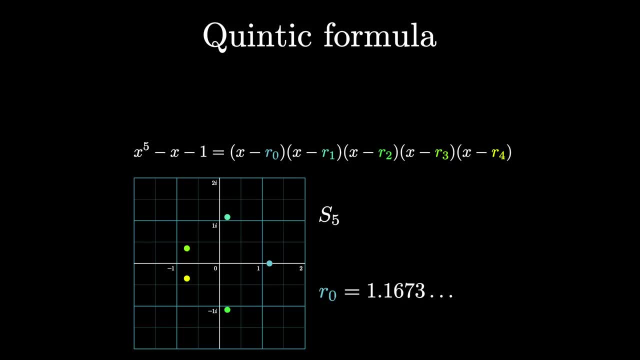 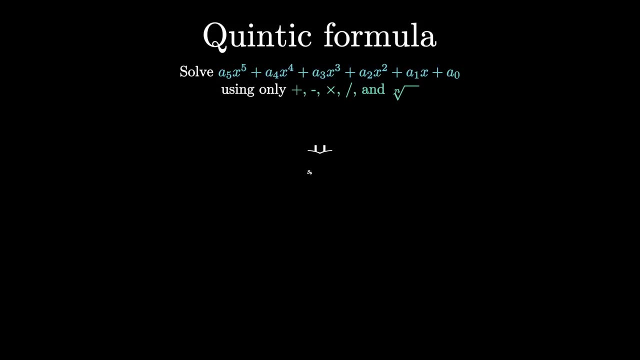 Well, if you're wondering what that proof actually looks like, it involves showing that if there were some kind of mythical quintic formula, something which uses only radicals and the basic arithmetic operations, it would imply that the permutation group on five elements decomposes into a special kind of simple group known fancifully as the cyclic groups of prime. 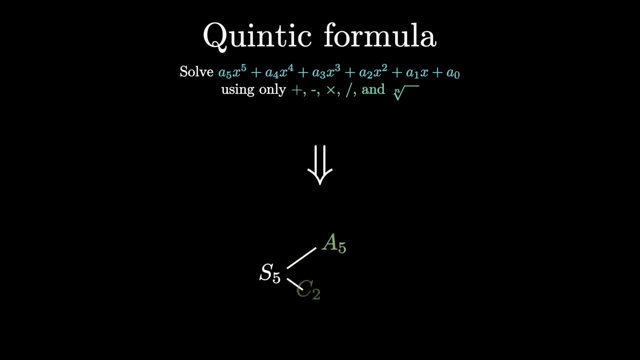 order, But the actual way that this breaks down involves a different kind of simple group, a different kind of atom, one which polynomial solutions built from radicals would never allow. That is a super high-level description, of course, with about a semester's worth of details missing. 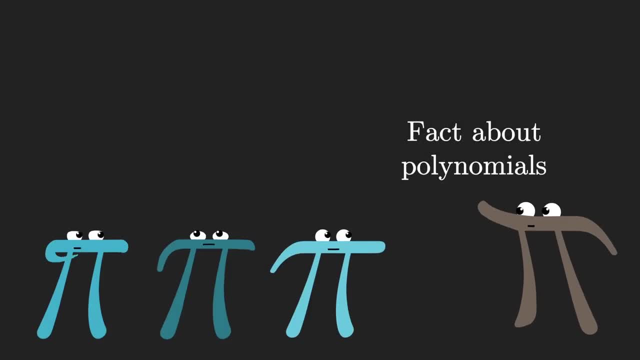 but the point is that you have this really not obvious fact about a different part of math whose solutions come from finding the atomic structure of a certain group. This is one of many different examples where understanding the nature of these simple groups, these atoms, actually matters outside of group theory. 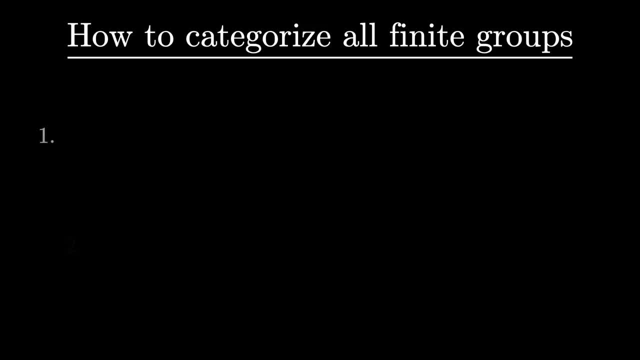 The task of categorizing all finite groups breaks down into two steps: One, find all the simple groups and two, find all of the ways to combine them. The first question is like finding the periodic table, and the second is a bit like doing all of chemistry thereafter. 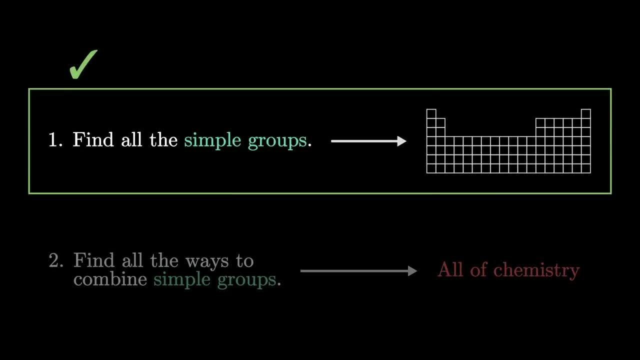 The good news is that mathematicians have found all of the finite simple groups. Well, more pertinent is that they proved that the ones that they found are in fact all the ones out there. It took many decades, tens of thousands of dense pages of advanced math. 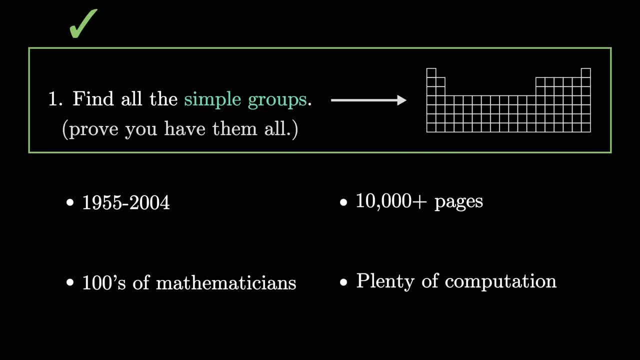 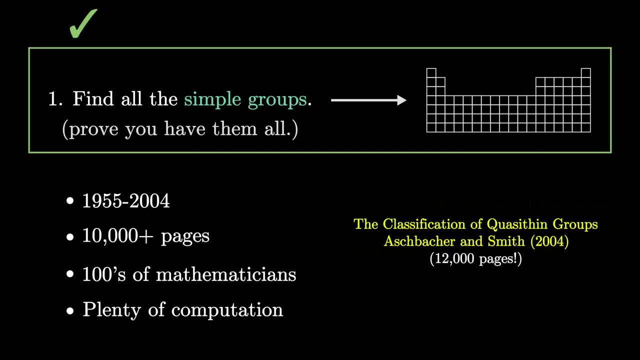 hundreds of some of the smartest minds out there and significant help from computers. But by 2004,, with a culminating 12,000 pages to tie up the loose ends- there was a definitive answer. Many experts agree this is one of the most monumental achievements in the history of math. 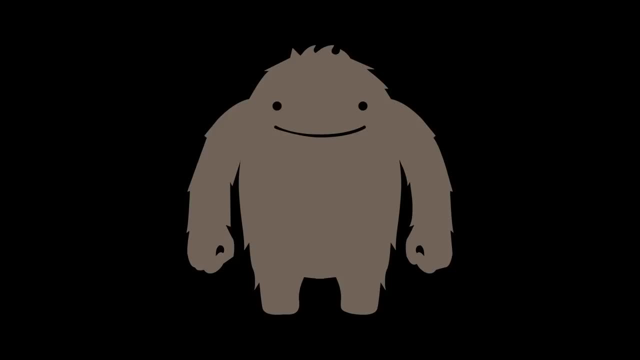 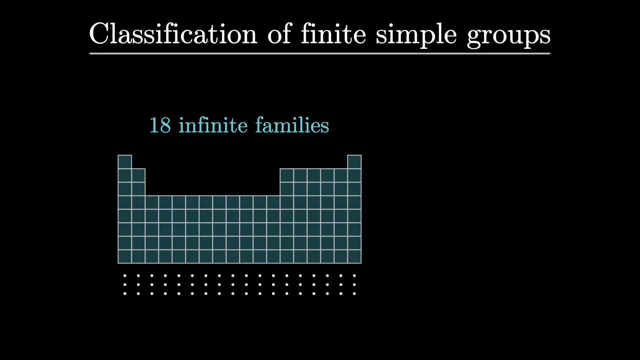 The bad news, though, is that the answer is absurd. There are 18 distinct, infinite families of simple groups, which makes it really tempting to lean into the whole periodic table, But groups are stranger than chemistry, because there are also these 26 simple groups that are just left over. 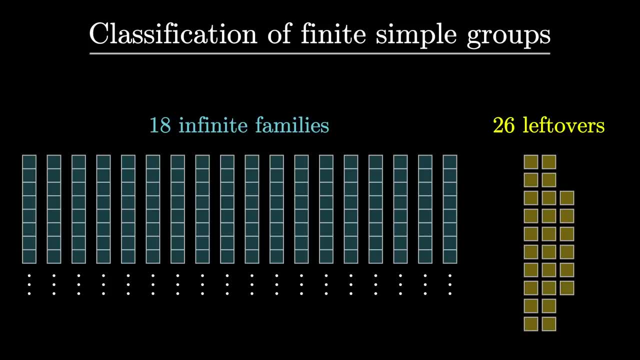 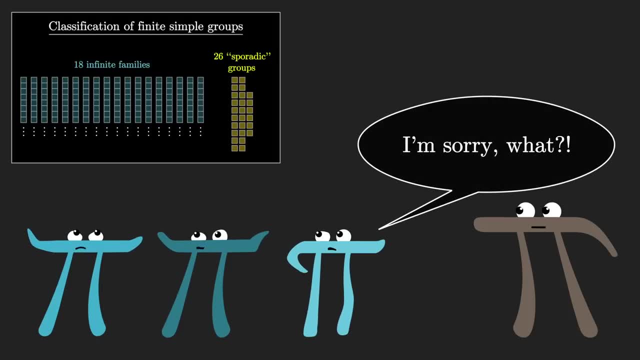 They don't fit the other patterns. These 26 are known as the sporadic groups. That a field of study rooted in symmetry itself has such a patched-together fundamental structure is well, I mean, it's just bizarre. It's like the universe was designed by committee. 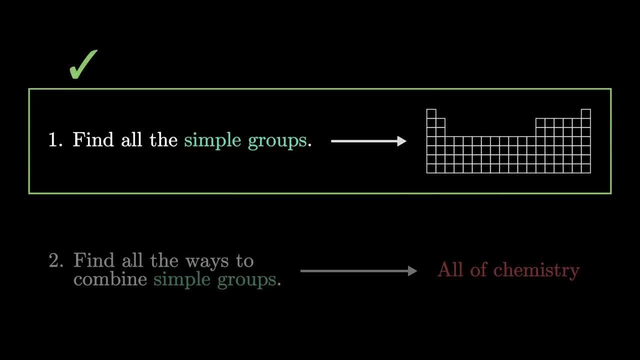 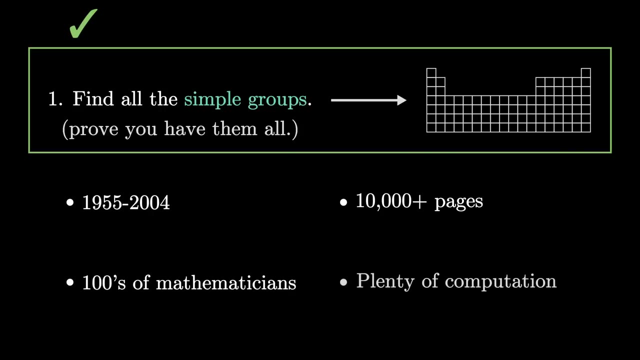 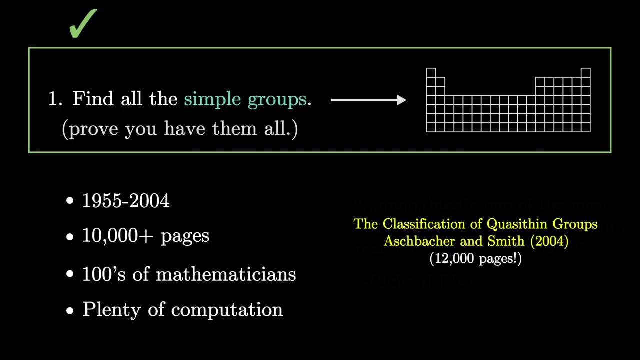 The good news is that mathematicians have found all of the finite simple groups. Well, more pertinent is that they proved that the ones they found are, in fact, all the ones out there. It took many decades, tens of thousands of dense pages of advanced math, hundreds of some of the smartest minds out there, and significant help from computers. But by 2004, with a culminating 12,000 pages to tie up the loose ends, there was a definitive answer. 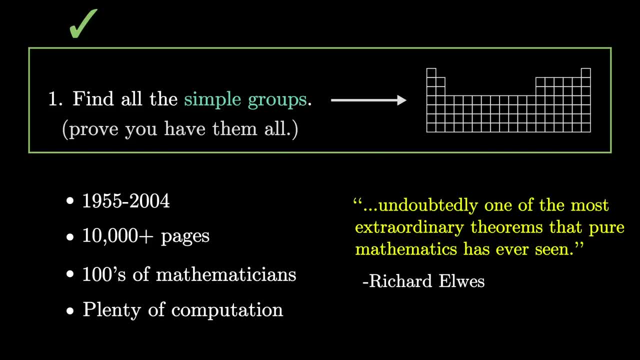 Many experts agree, this is one of the most monumental achievements in the history of math. 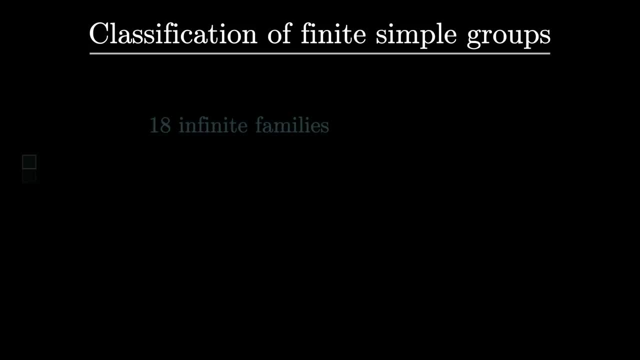 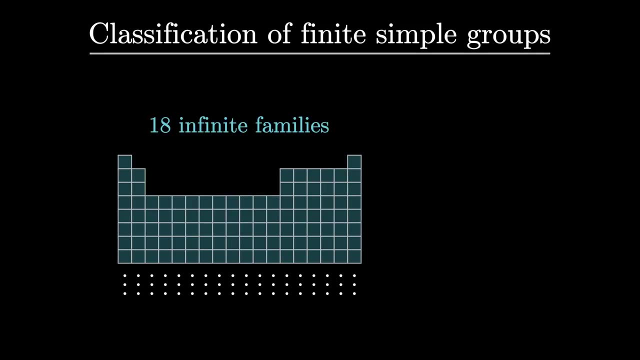 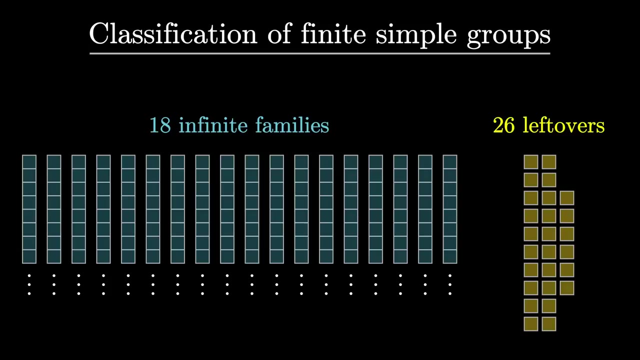 The bad news, though, is that the answer is absurd. There are 18 distinct infinite families of simple groups, which makes it really tempting to lean into the whole periodic table analogy. But groups are stranger than chemistry, because there are also these 26 simple groups that are just left over. They don't fit the other patterns. These 26 are known as the sporadic groups. 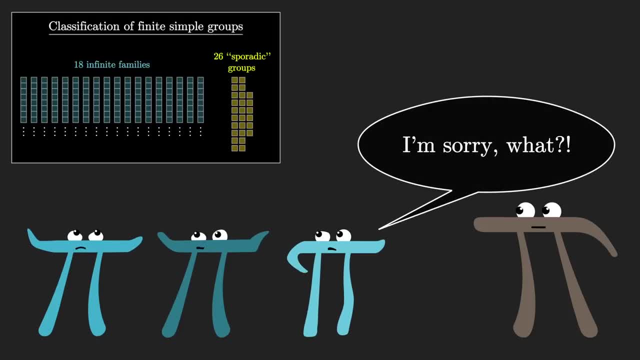 And their symmetry itself is such a patched together fundamental structure, it is… well, I mean, it's just bizarre. It's like the universe was designed by committee. 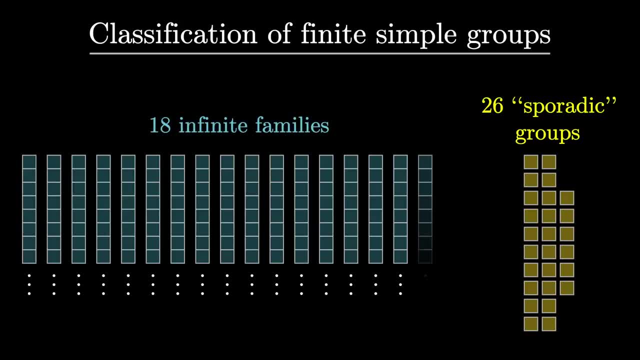 If you're wondering what we mean by an infinite family, examples might help. One such family of simple groups includes all of these cyclic groups with prime order. 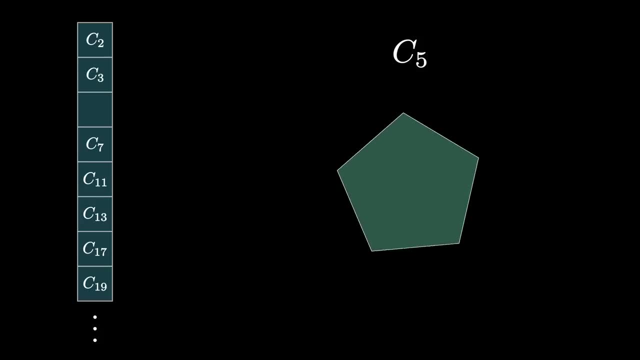 These are essentially the symmetries of a regular polygon with a prime number of sides, but where you're not allowed to flip the polygon over. Another of these infinite families 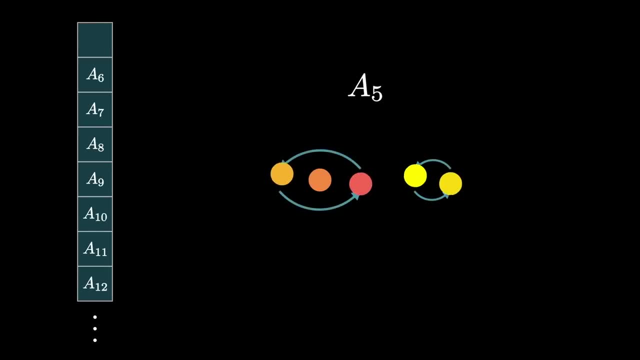 is very similar to the permutation groups we saw earlier. earlier, but there's the tiniest constraint on how they're allowed to shuffle n items. 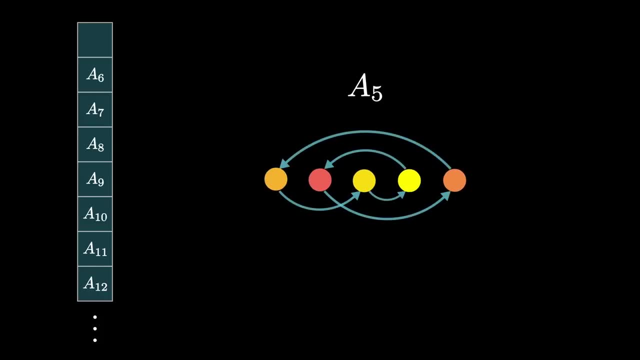 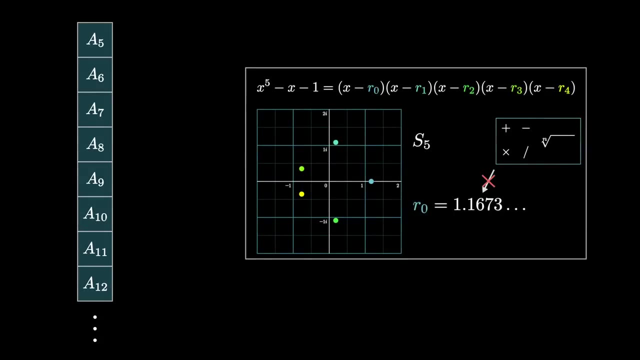 If they act on 5 or more elements, these groups are simple. Which incidentally is heavily related to why polynomials with degree 5 or more have solutions that can't be written down using radicals. 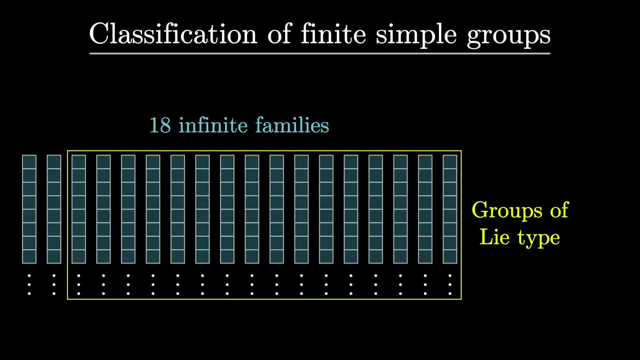 The other 16 families are notably more complicated, and I'm told that there's at least a little ambiguity in how to organize them into cleanly distinct families without overlap, but what 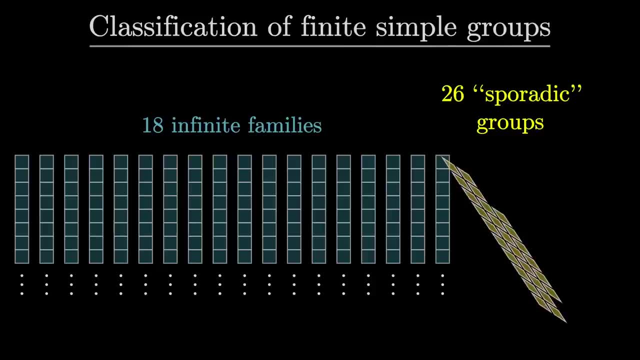 everybody agrees on is that the 26 sporadic groups stand out as something very different. The largest of these sporadic groups is known, thanks to John Conway, as the monster group, and its size is the number I mentioned at the start. 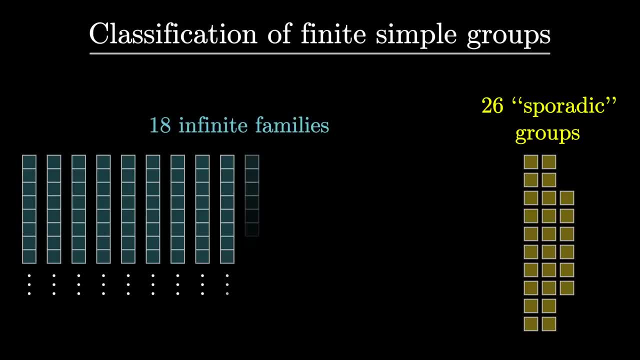 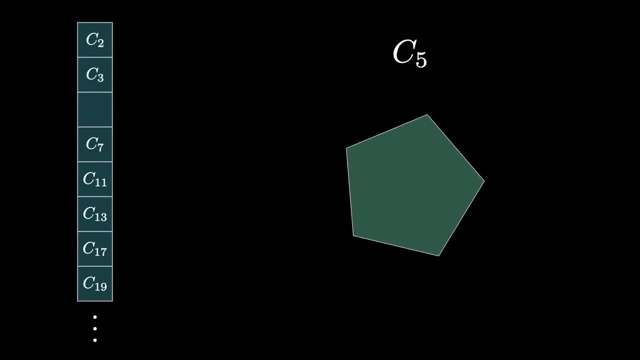 If you're wondering what we mean by an infinite family, examples might help. One such family of simple groups includes all of these cyclic groups with prime order. These are essentially the symmetries of a regular polygon with a prime number of sides. 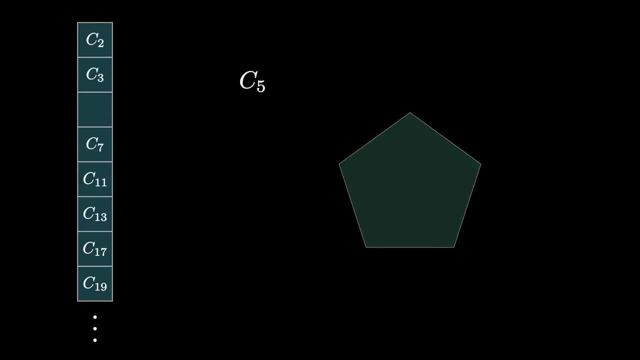 but where you're not allowed to flip the polygon over. Another of these infinite families is very similar to the permutation groups that we saw earlier, but there's the tiniest constraint on how they're allowed to shuffle n items. If they act on five or more elements, these groups are simple. 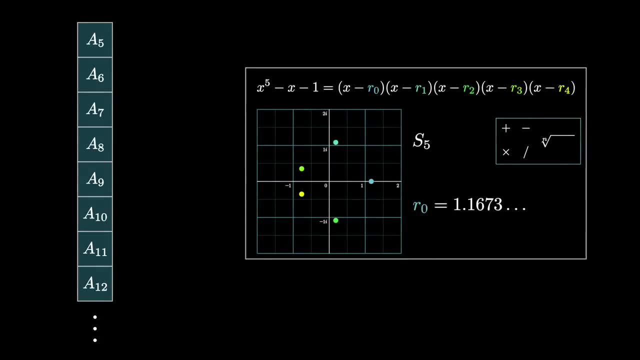 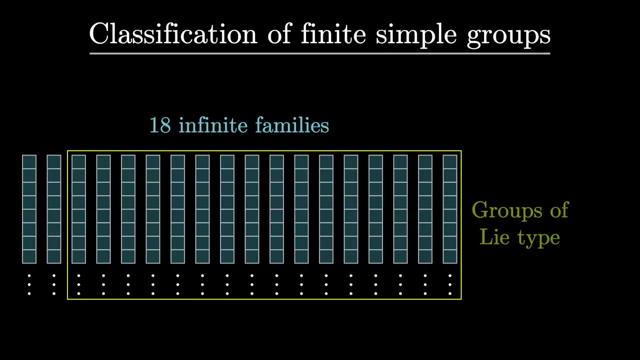 Which, incidentally, is heavily related to why polynomials with degree five or more have solutions that can't be written down using radicals. The other 16 families are notably more complicated, and I'm told that there's at least a little ambiguity in how to organize them into cleanly distinct families without overlap. 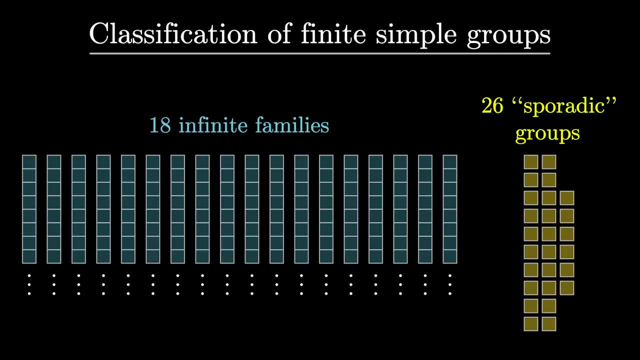 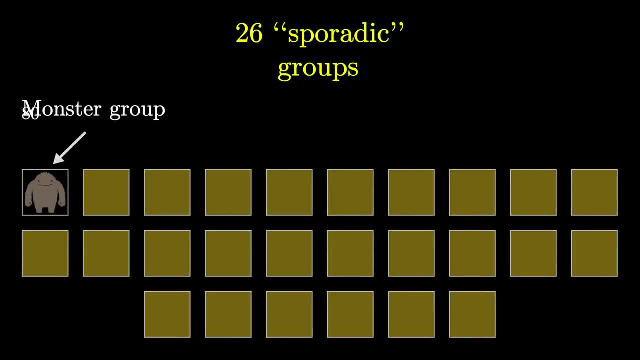 but what everybody agrees on is that the 26 sporadic groups stand out as something very different. The largest of these sporadic groups is known, thanks to John Conway, as the monster group, and its size is the number I mentioned at the start. 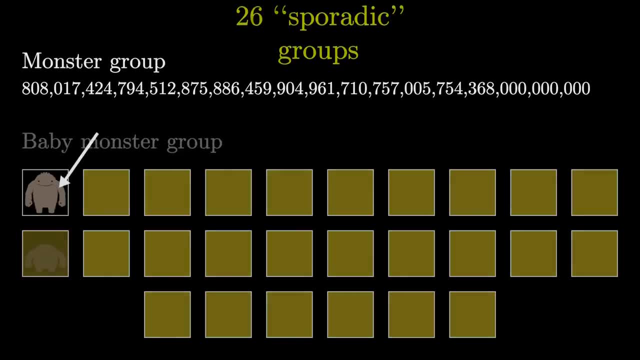 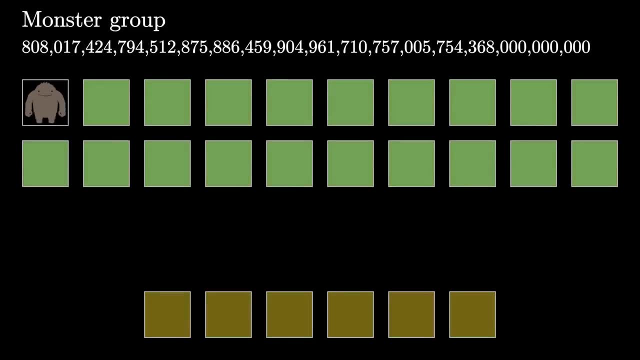 The second largest- and I promise this isn't a joke- is known as the baby monster group. Together with the baby monster, 19 of these sporadic groups are, in a certain sense, children of the monster, and Robert Gries called these 20 the happy family. 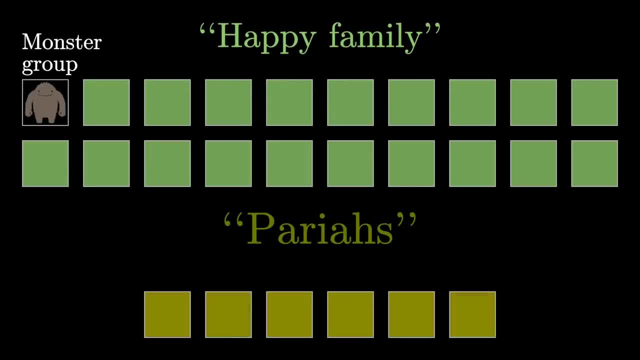 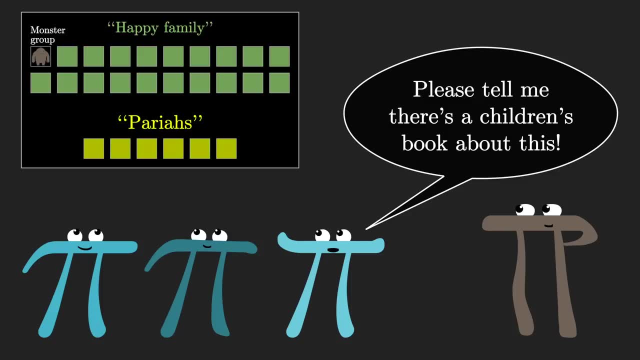 He also called the other six which don't even fit that pattern, the pariahs, As if to compensate for how complicated the underlying math here is. the experts really let loose on their whimsy while naming things. Let me emphasize: having a group which is big is not that big a deal. 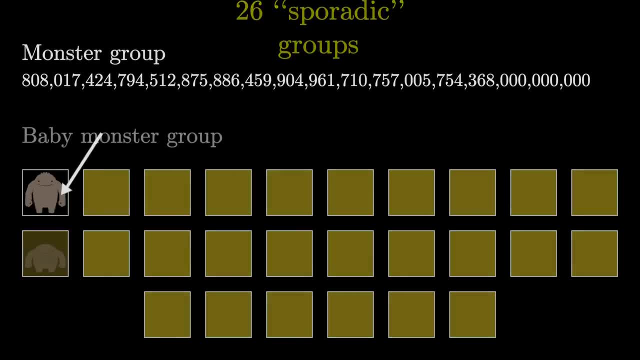 The second largest, and I promise this isn't a joke, is known as the baby monster group. Together with the baby monster, 19 of these sporadic groups are in a certain sense children 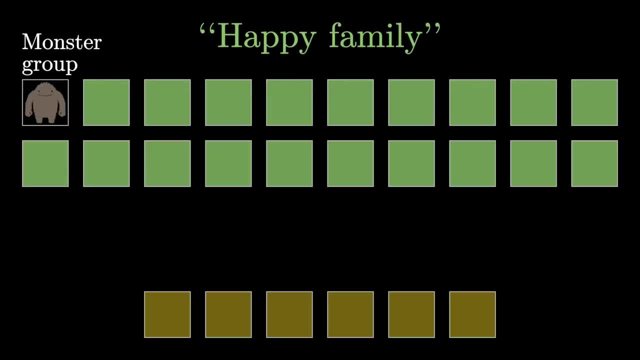 of the monster, and Robert Gries called these 20 the happy family. He also called the other 6, which don't even fit there, the happy family. 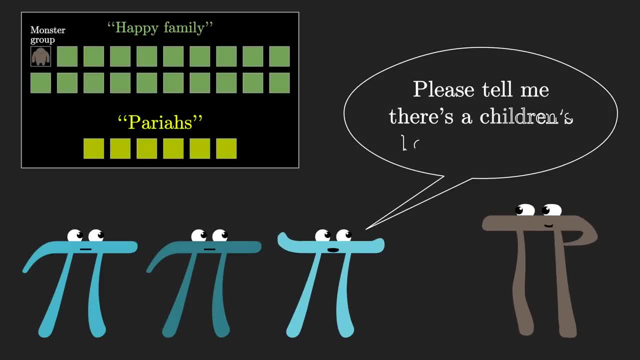 And the last one is known as the pariahs. As if to compensate for how complicated the underlying math here is, the experts really 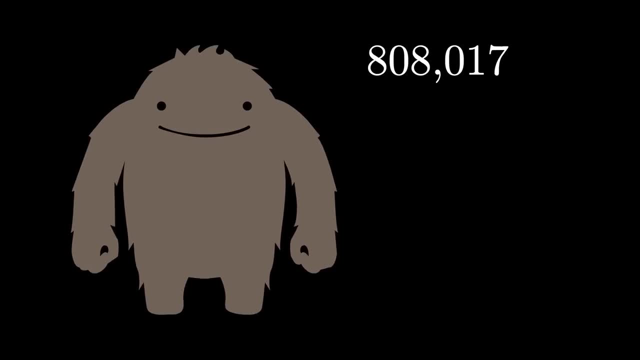 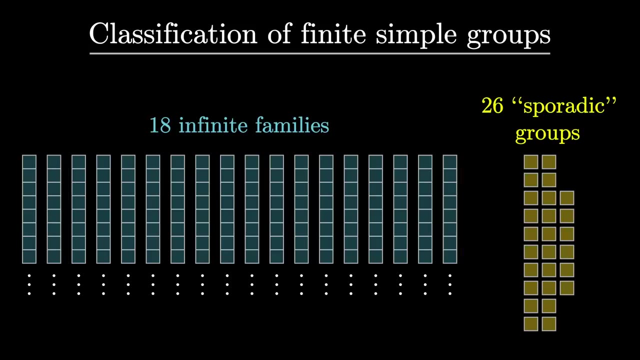 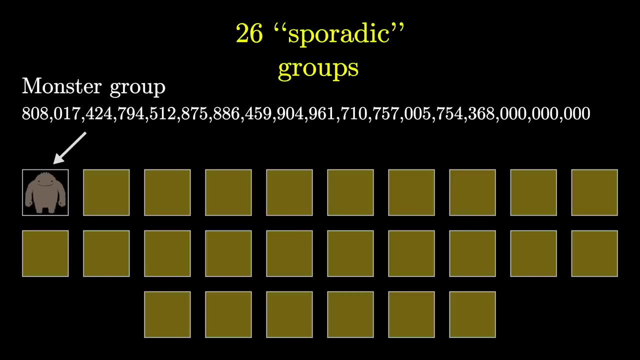 let loose on their whimsy while naming things. Let me emphasize, having a group which is big is not that big a deal, but the idea that one of the fundamental building blocks for one of the most fundamental ideas in math comes in a collection that just abruptly stops around 8x10 to the 53, that's weird. 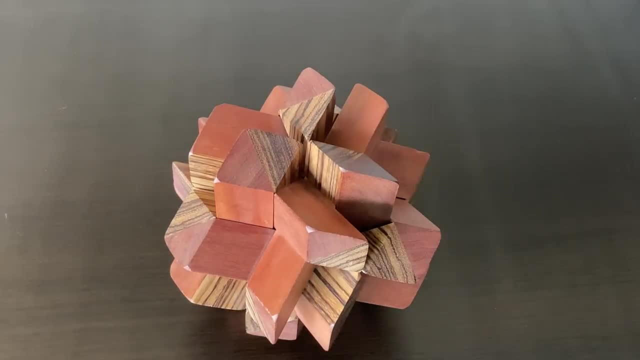 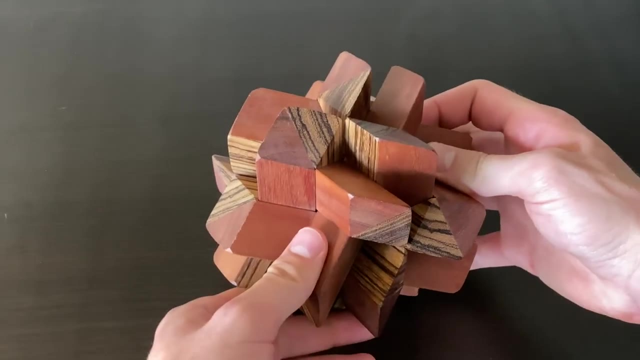 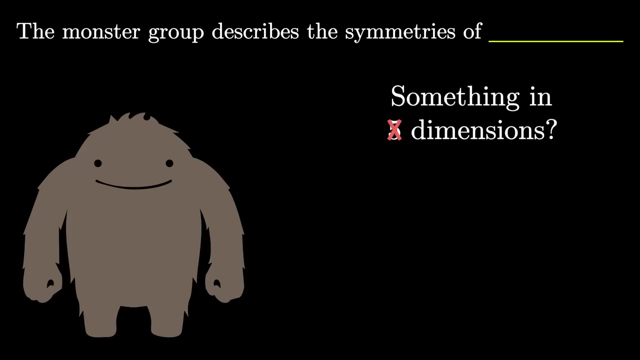 Now at this point, given that I introduced groups as symmetries, a collection of actions, you might wonder what it is that the monster acts on. What object does it describe the symmetries of? Well there is an answer, but it doesn't fit into 2 or 3 dimensions to draw, nor does it fit into 4 or 5. 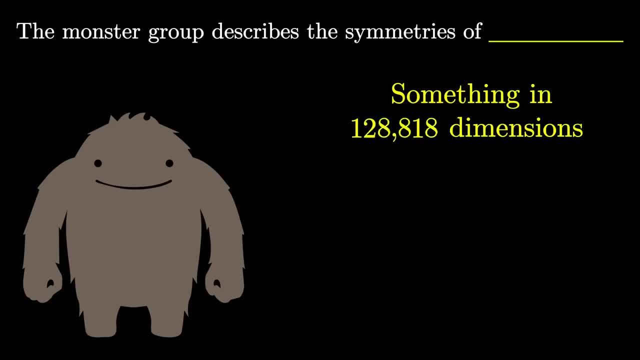 Instead, to see what the monster acts on, we would have to jump up to...wait for it...196,883 dimensions. 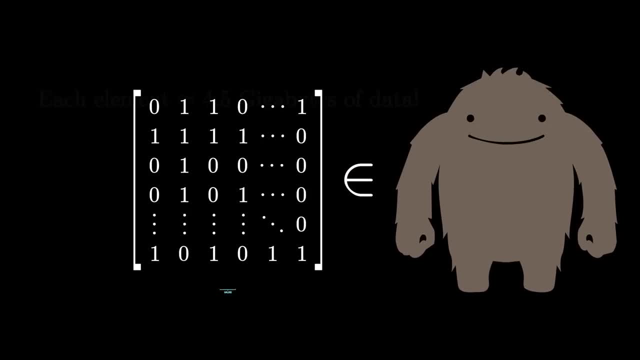 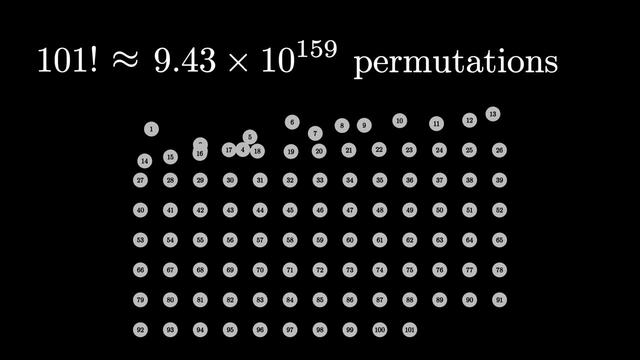 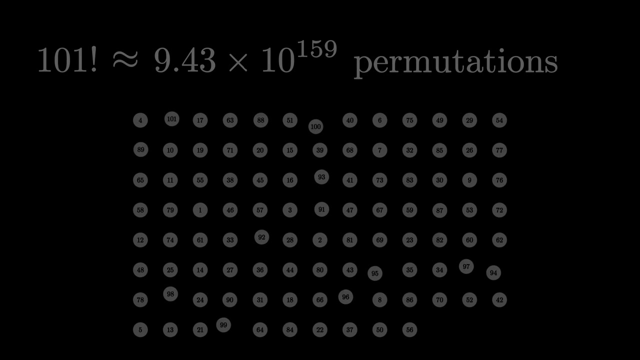 Just describing one of the elements of this group takes about 4 gigabytes of data, even though plenty of groups that are way bigger have a much smaller computational description. The permutation group on 101 elements was, if you'll recall, dramatically bigger, but we can describe each one of its elements with very little data, for example a list of 100 numbers. 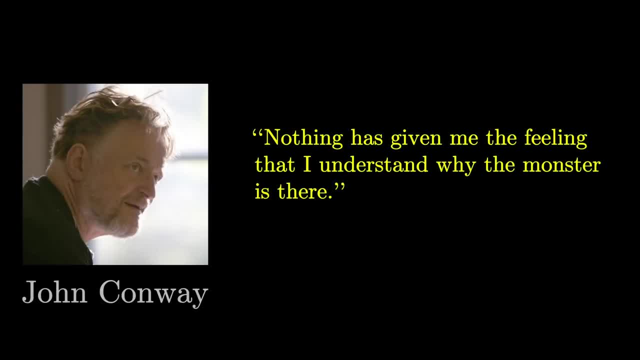 No one really understands why the sporadic groups, and the monster in particular, are there. Maybe in a few decades there will be a clearer answer. Maybe one of you will come up with it. 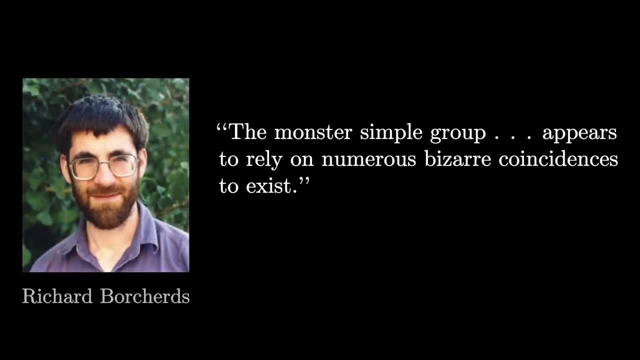 But despite knowing that they are deeply fundamental to math, and arguably to physics as well, a lot about them remains mysterious. 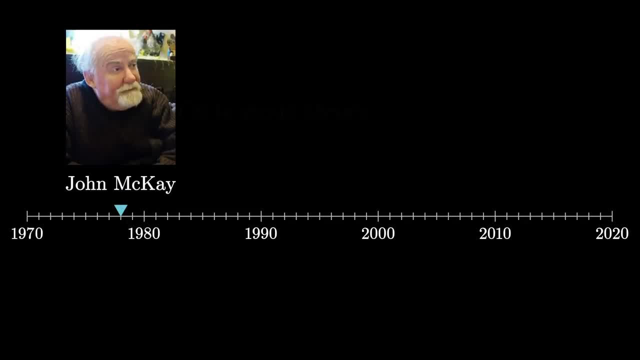 In the 1970s, mathematician John McKay was making a switch from studying group theory to an adjacent field, and he noticed that a number very similar to this 196,883 showed 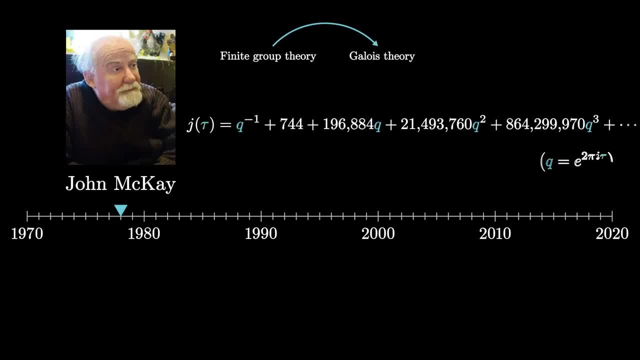 up in a completely unrelated context. Or at least almost. A number one bigger than this was in the series expansion of a fundamental function in a totally different part of math. 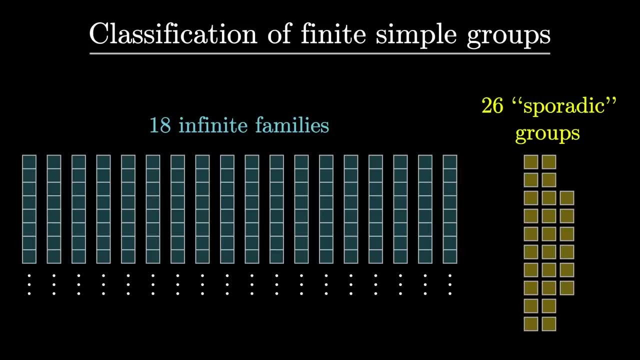 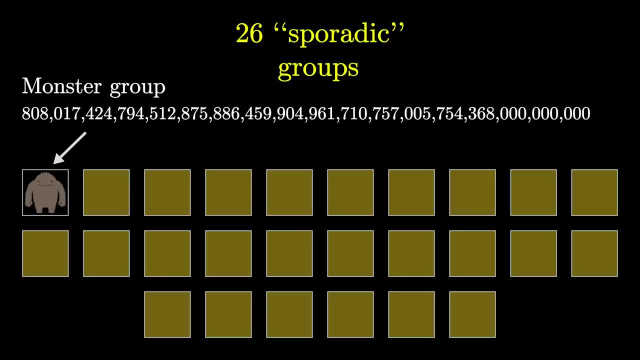 but the idea that one of the fundamental building blocks for one of the most fundamental ideas in math comes in a collection that just abruptly stops around 8 times 10 to the 53, that's weird Now at this point, given that I introduced groups as symmetries. a collection of actions. 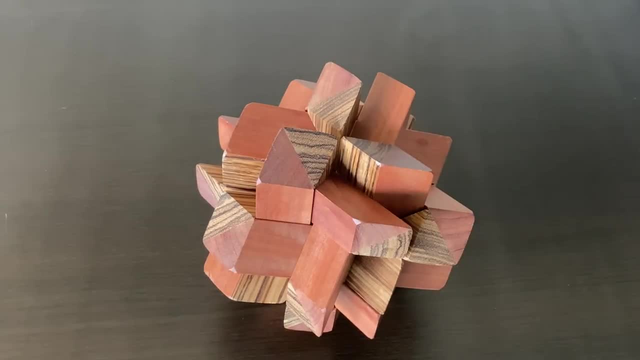 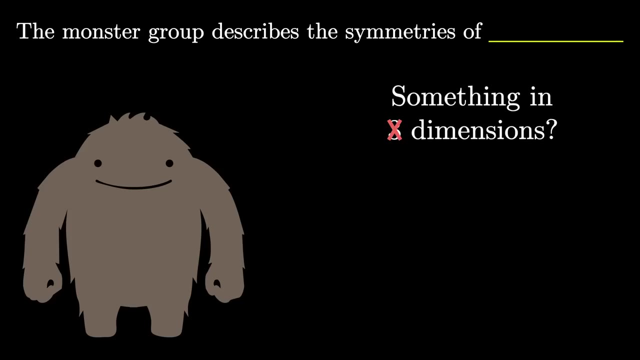 you might wonder what it is that the monster acts on. What object does it describe the symmetries of? Well, there is an answer. but it doesn't fit into two or three dimensions to draw, nor does it fit into four or five. 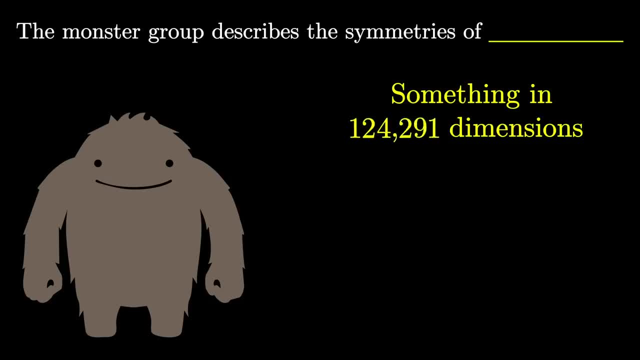 Instead, to see what the monster acts on, we would have to jump up two, wait for it and see what it does. 196,883 dimensions- Just describing one of the elements of this group- takes about 4 gigabytes of data. 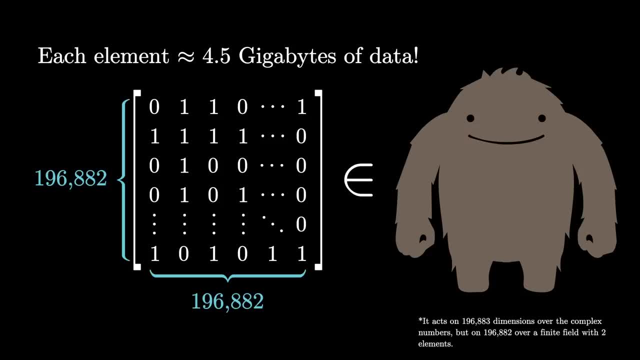 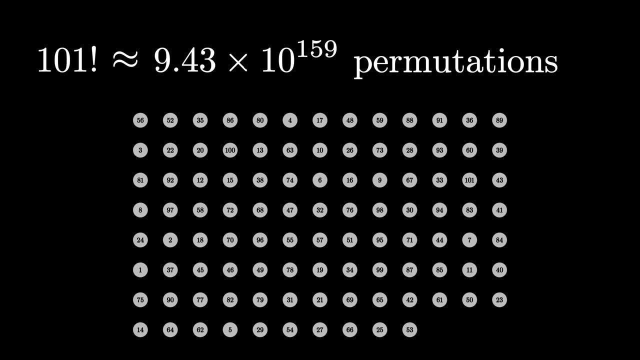 even though plenty of groups that are way bigger have a much smaller computational description. The permutation group on 101 elements was, if you'll recall, dramatically bigger, but we can describe each one of its elements with very little data, for example a list of 100 numbers. 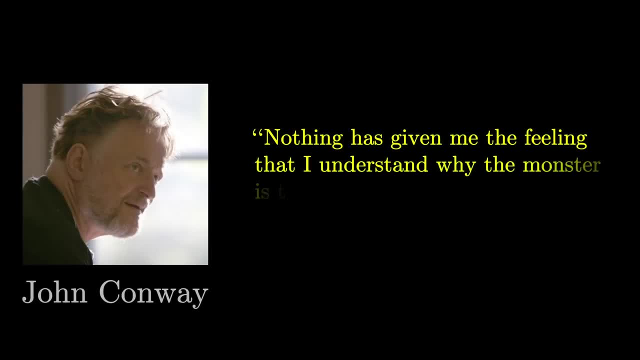 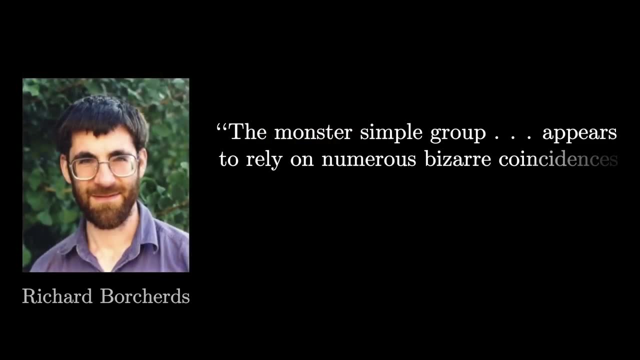 No one really understands why the sporadic groups, and the monster in particular, are there. Maybe in a few decades there will be a clearer answer, maybe one of you will come up with it, But despite knowing that they are deeply fundamental to math. 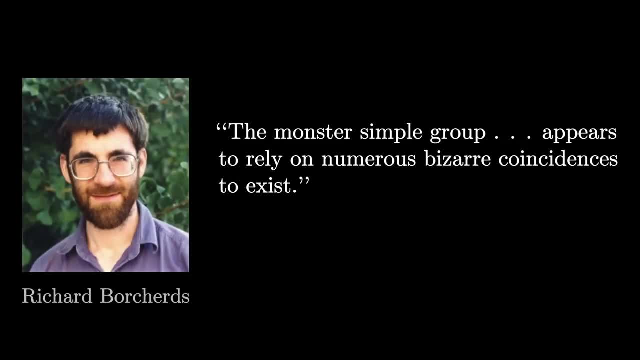 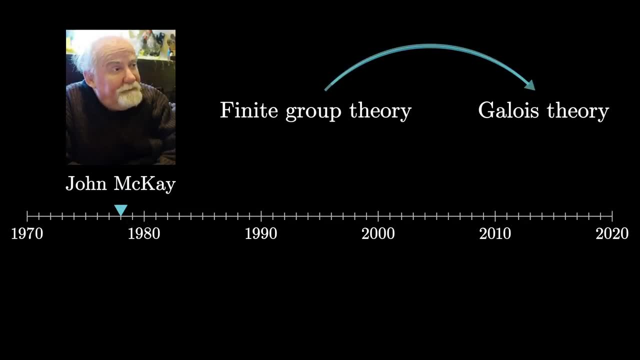 and arguably to physics as well. a lot about them remains mysterious. In the 1970s, mathematician John McKay was making a switch from studying group theory to an adjacent field, and he noticed that a number very similar to this- 196,883,. 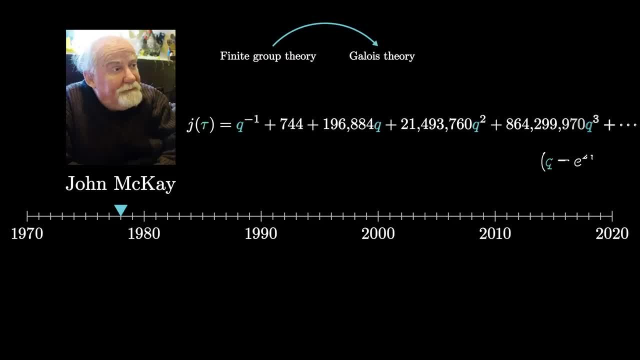 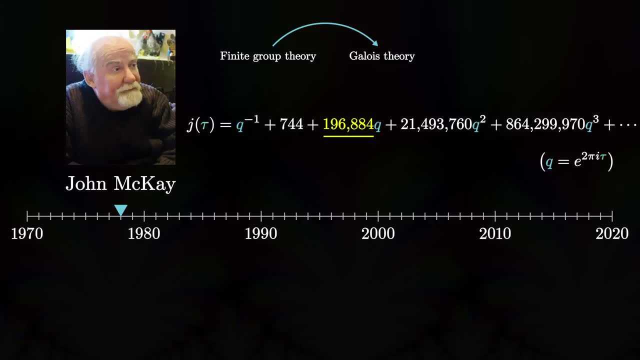 showed up in a completely unrelated context, Or at least almost A number one bigger than this was in the series expansion of a fundamental function in a totally different part of math relevant to these things called modular forms and elliptic functions. Assuming that this was more than a coincidence seemed crazy. 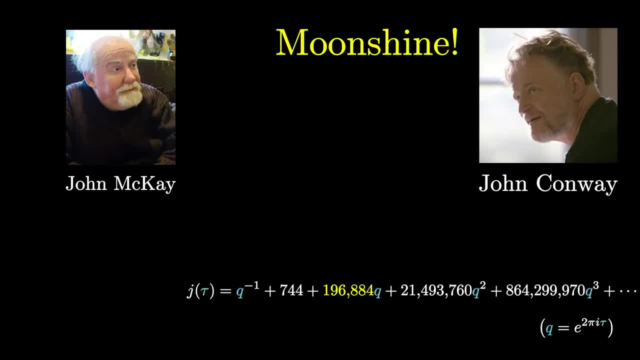 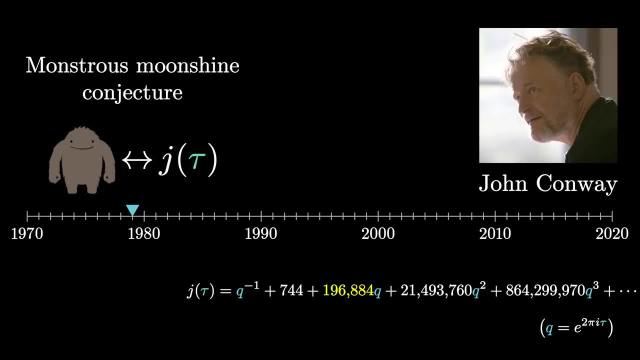 enough that it was playfully deemed moonshine by John Conway. But after more numerical coincidences like this were noticed, it gave rise to what became known as the monstrous moonshine conjecture. Whimsical names just don't stop. This was proved by Richard Borchards in 1992, solidifying a connection between 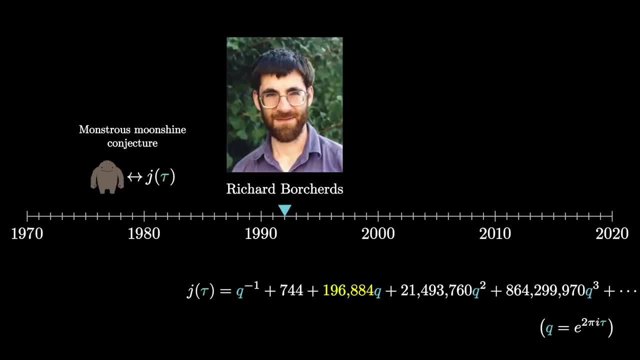 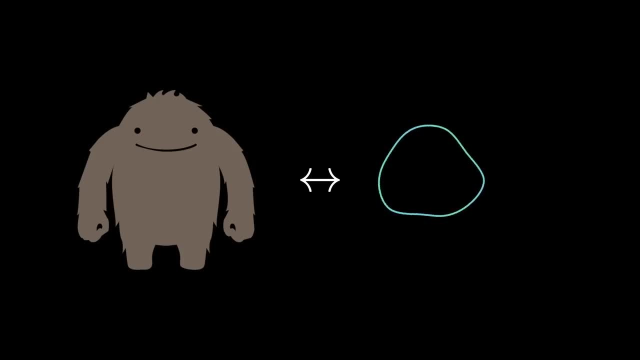 very different parts of math that at first glance seemed crazy. Six years later, by the way, he won the Fields Medal, in part for the significance of this proof, And related to this, moonshine is a connection between the monster and string theory. 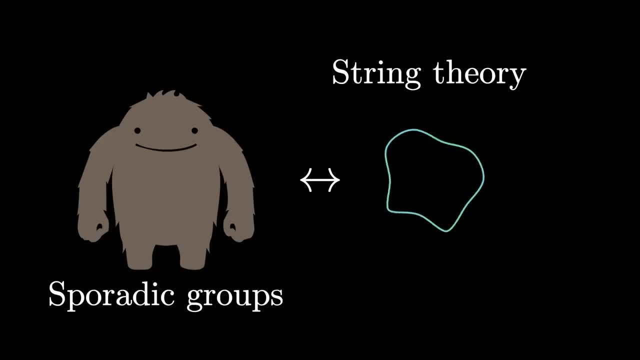 Maybe it shouldn't come as a surprise that something that arises from symmetry itself is relevant to physics. but in light of just how random the monster seems at first glance, this connection still elicits a double take To me. the monster and its absurd size is a nice reminder that fundamental objects 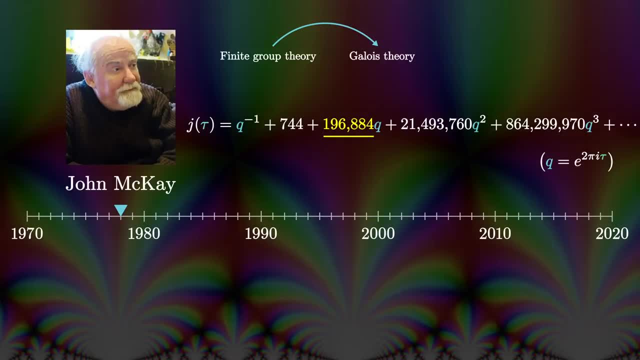 Relevant to these things in general. These things called modular forms, and elliptic functions. 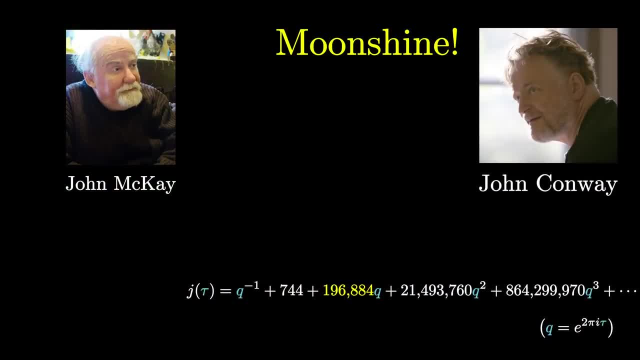 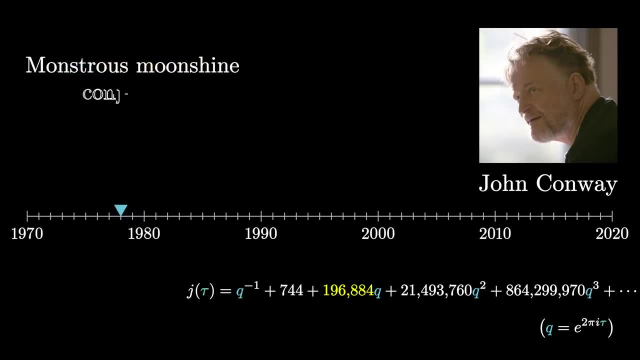 Assuming that this was more than a coincidence seemed crazy, enough that it was playfully deemed moonshine by John Conway. But after more numerical coincidences like this were noticed, it gave rise to what became known as the monstrous moonshine conjecture. Whimsical names just don't stop. 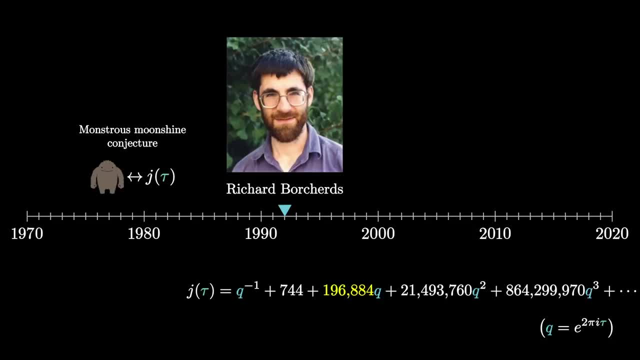 This was proved by Richard Borchardt's in 1992, solidifying a connection between very different parts of math that at first glance seemed crazy. 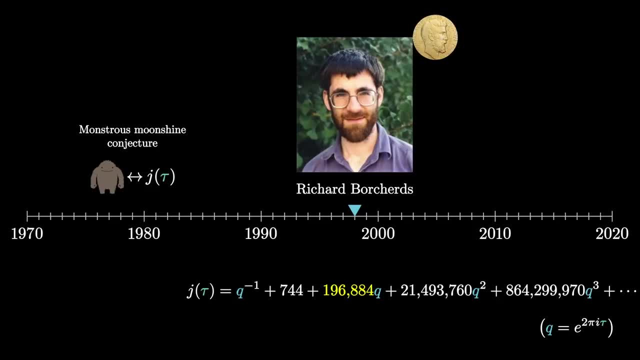 Six years later, by the way, he won the Fields Medal. In part for the significance of this proof. 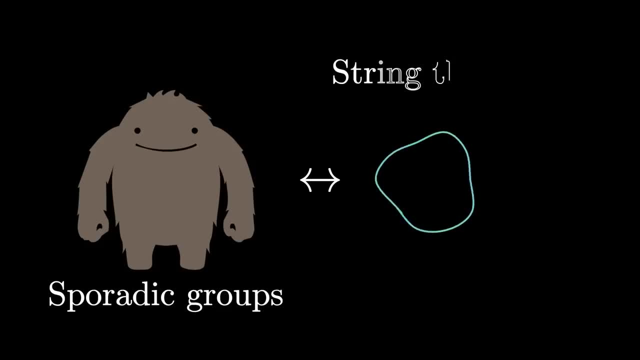 And related to this moonshine is a connection between the monster and string theory. Maybe it shouldn't come as a surprise that something that arises from symmetry itself is relevant to physics, but in light of just how random the monster seems at first glance, 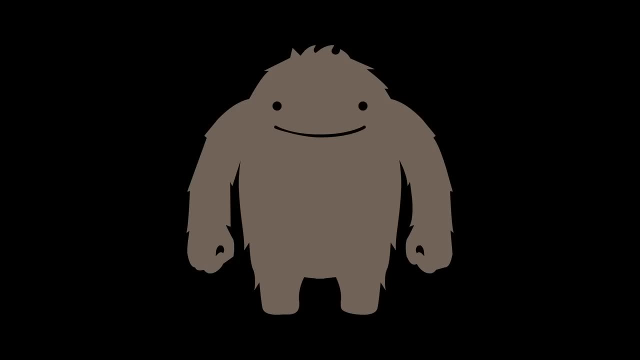 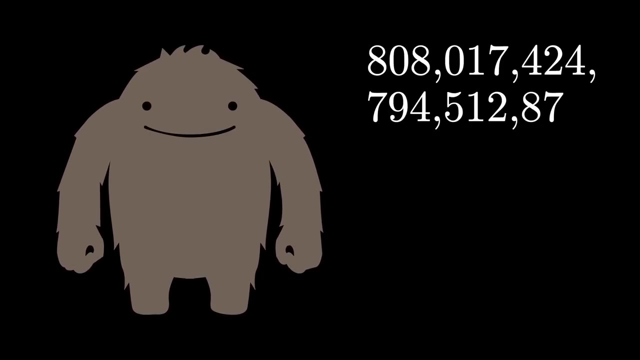 this connection still elicits a double take. To me, the monster and its absurd size is a nice reminder that fundamental objects are not necessarily simple. The universe doesn't really care if its final answers look clean. 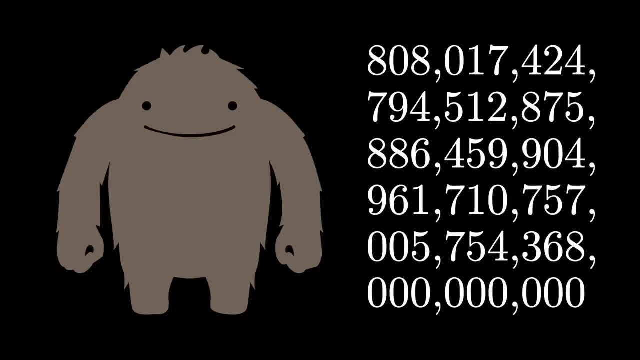 They are what they are by logical reasoning. They are what they are by mathematical necessity, with no concern over how easily we'll be able to understand them. 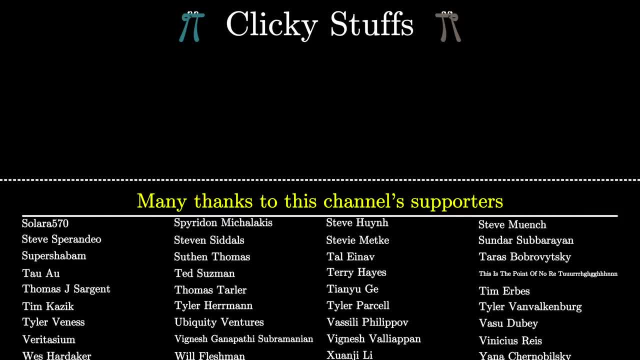 They are what they are by mathematical necessity, with no concern over how easily we'll be able to understand them. Okay, so let's start. 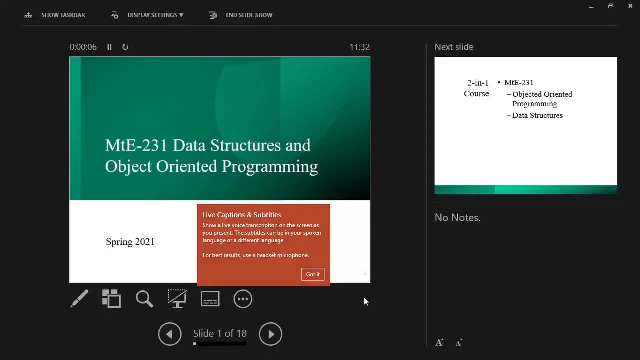 Okay, so this course, as I hope you already know, like it is data structures and object-oriented programming. Now, it is a combo course, like it is a combination of two courses. If you have friends in, say, computer systems or computer science, so they study this course as two separate courses. They first study object-oriented programming in a lot of detail, and then they go and study data structures. So, in our case, like we only have this one course, and we try to cover as much ground as possible in this particular course. Why study object-oriented programming and data structures? So, you have only, like you have just studied computer programming, and that is fairly fundamental, basic programming. This is slightly more advanced, like wherever you left in computer programming in this course, we start from there.